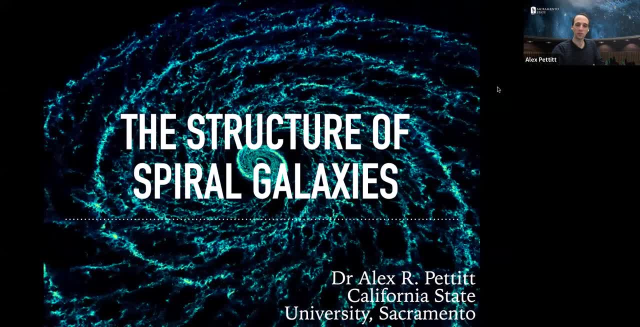 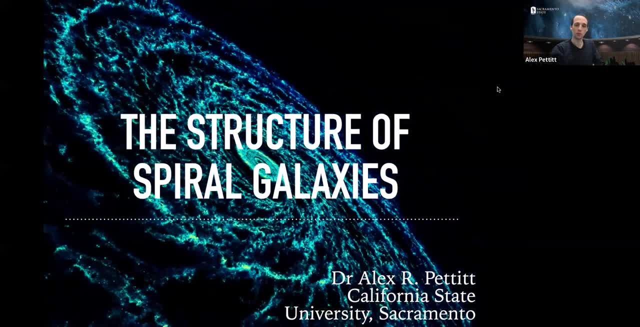 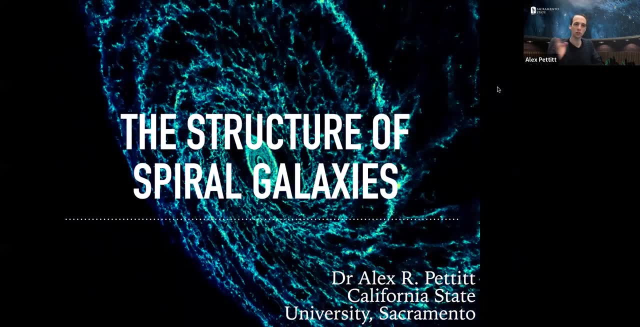 And I've got some simulations spinning around. I'm going to talk to you in a bit more detail about this later on. If you've got any questions- I don't know what your normal format here- I'm happy to take questions during the talk if you'd like to do that, or I'm also happy to field them at the end, if you prefer. 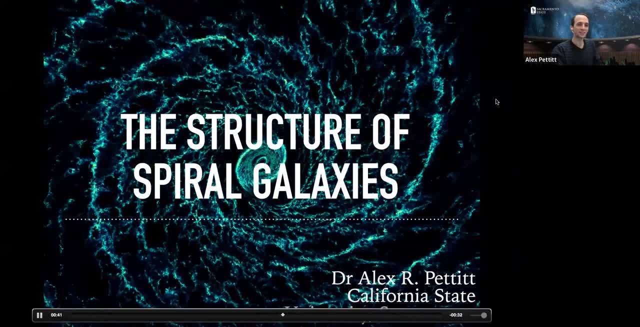 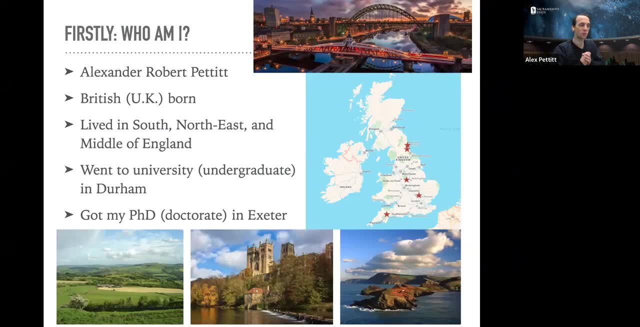 I don't know what you've organized, but either is fine with me. So, as I already said, I'm Alex. I'd like to give a bit of an introduction to myself first, before we start. You might be able to tell from my voice that I'm British. 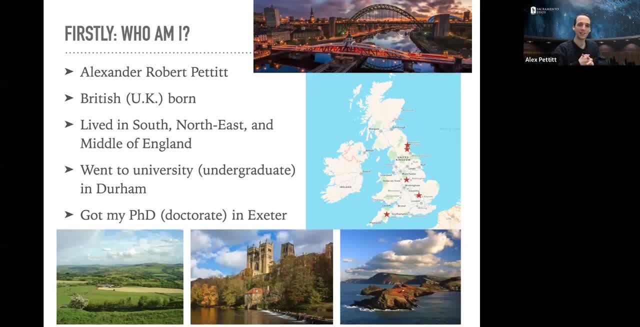 I spent my undergraduate and postgraduate days in the United Kingdom. I've moved up and down the country a lot, for my different studies lived in places like Exeter and Durham. they're not super well known places, but it's taken me north and south and to the center of the country- all sorts of different locales. 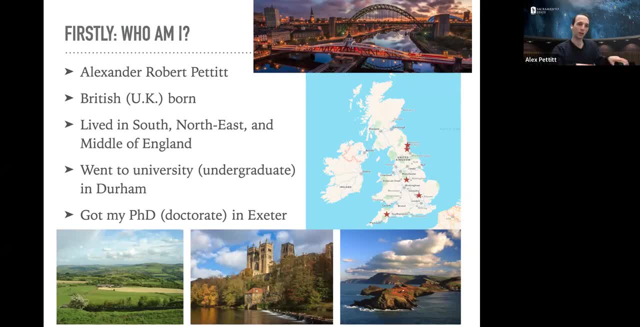 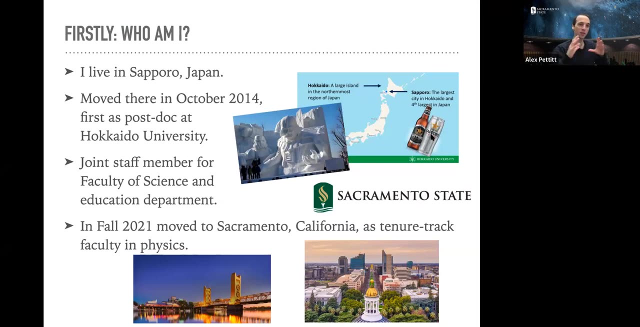 But you might know a little bit about academia and that you don't tend to stay in one place for very long, so researchers move around a lot. So once I finished my studies, I moved over To Japan, a place called Sapporo. you might have heard of this if you've ever seen Sapporo beer before, so it's famous for the beer and for a lot of snow. 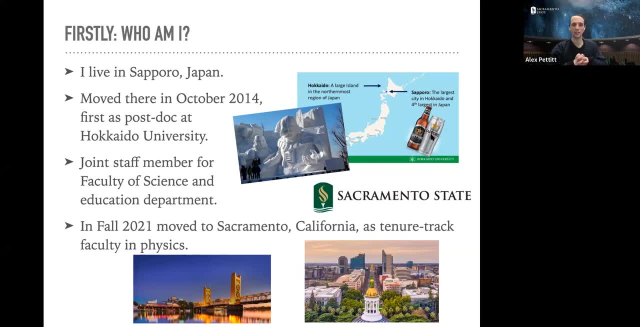 And I lived there for the better part of about six or seven years. I went there for a what's called a postdoc, so the first job you have after your PhD- and I had a short term professorship there as well, right towards students. 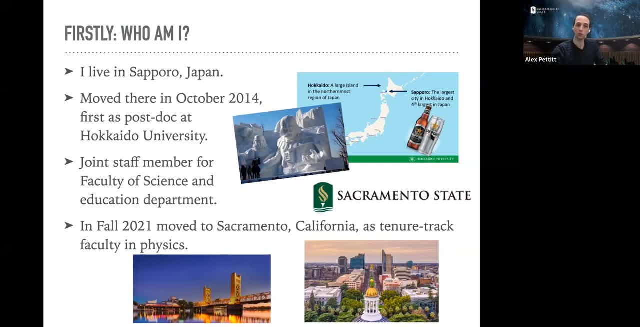 And after that fall of last year- should have been a fall of The year before that, but COVID is as COVID is- I moved to California, to Sacramento, which is where I am at the moment, and I'm a permanent faculty here teaching and doing research and all that other academic good stuff. 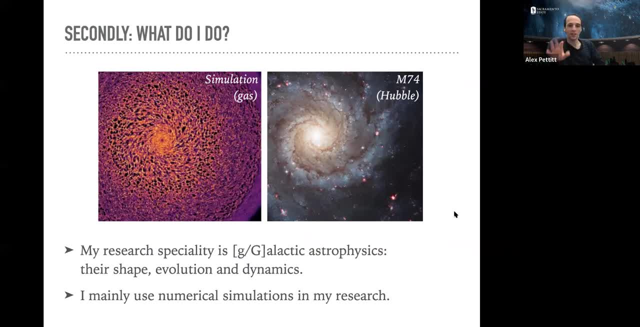 So today I'm going to talk to you about galaxies and the kind of work that I do, and I'm going to just tease it at the start a little bit with showing you. this on the left is a simulation of one of my galaxies here. 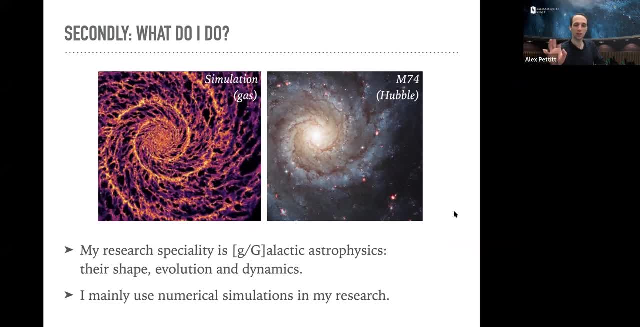 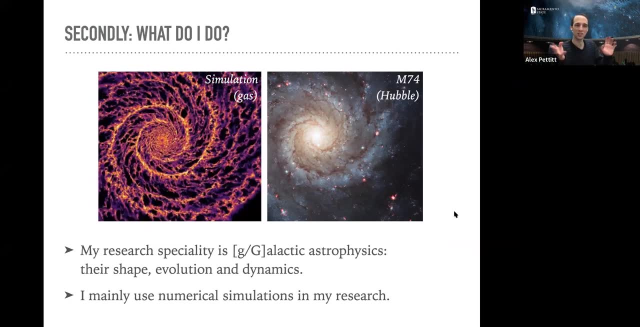 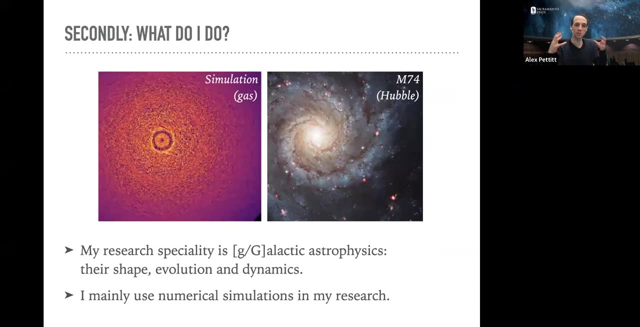 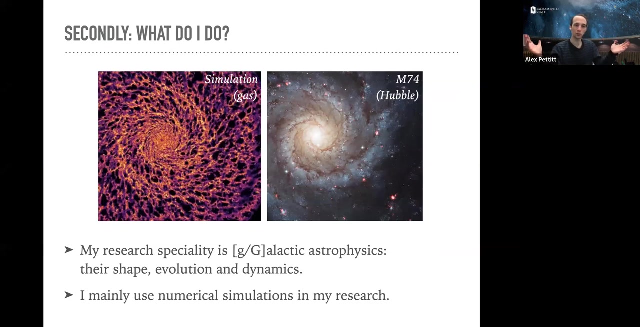 And on the right is a image of optical light, so visible light, coming from a galaxy called M7. It's not a not a very tantalizing name, but it's. a lot of galaxies have these numbers and letters names to them And I'll play that again just to show that a little bit clearer. So in my work I spent a lot of time making computers do experiments for me. So galaxies are very big, very old and very complicated objects so it's very hard to understand what they're doing. 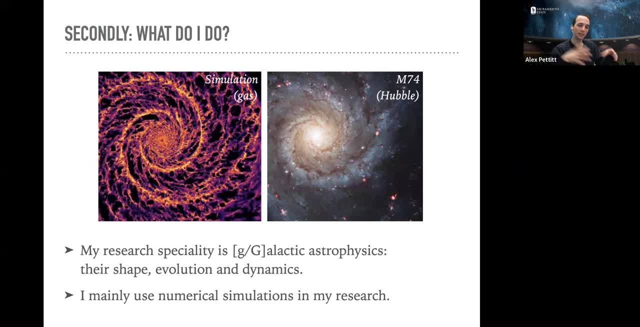 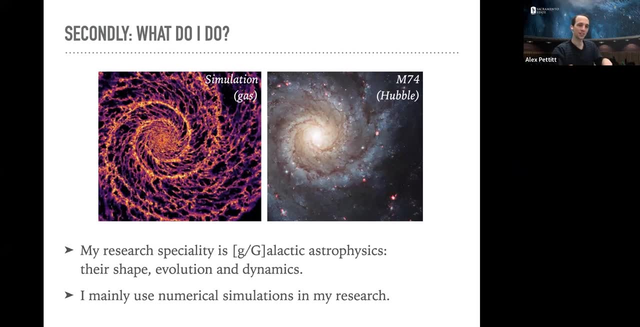 To make things a little bit easier. rather than just using telescope data all the time, we build little galaxies inside a computer And we can use those to study how the real things behave. So all sorts of advantages to this. have a lot more control over it. And we can try all different types of galaxies over and study them for millions and millions of years, whereas for the things in the night sky we have a lot less kind of control as to what we're looking at and it's a lot harder to delve into the nitty gritty details of what a galaxy is doing just through looking at it through a telescope. 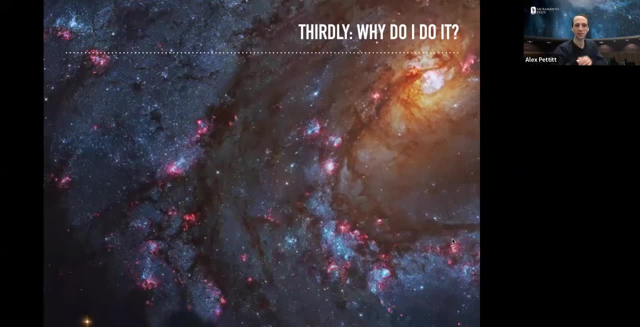 So why? why do we care about, about galaxies in the first place? Here's another beautiful picture of what we call a barred galaxy. So this long thing in the top right with the bar of the galaxy, this kind of orangey thing, the long 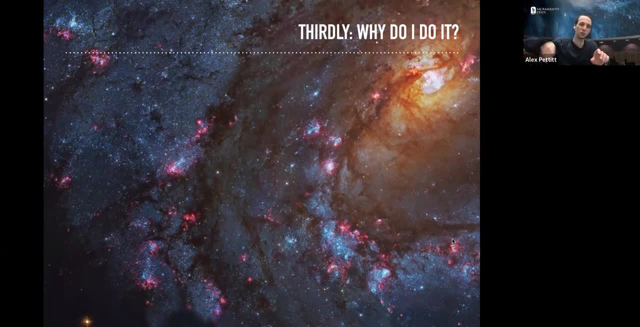 rectangular almost shape, and these beautiful things coming out of it from the center are called spiral arms. I'll talk about this in a bit more detail later on. But but why do we care about this thing? Why should you study this? Why should I study this? Why am I spending taxpayers money on looking at this thing? 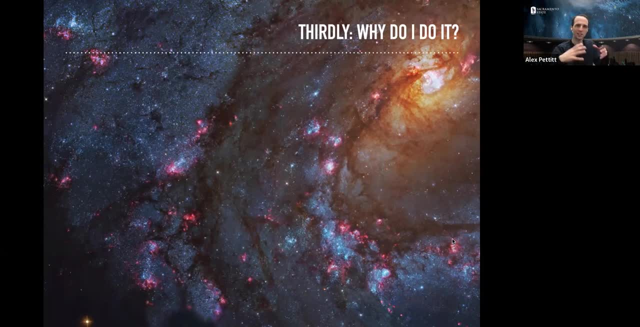 So a galaxy is kind of like an engine, In a sense. takes in fuel. In this case it's gas, effectively Hydrogen, helium, that kind of stuff. Galaxies are full of it. About 10% of their mass is gas. And they take in this gas and they transform it into stars over a process that can take a few million years or so, And in doing so they are kind of like a little factory or an engine. They take in this gas, they turn it away, do some physical processes on it and they spit stars out. 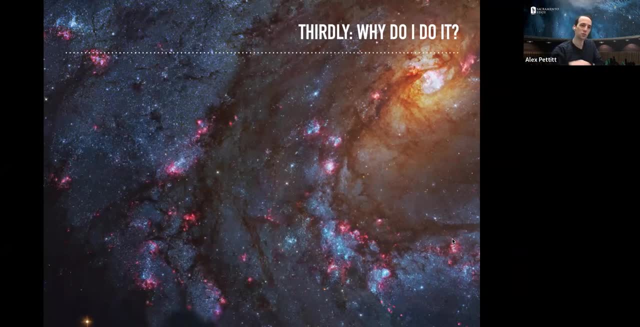 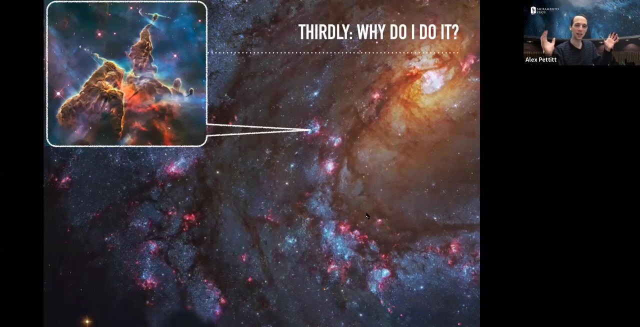 the other side. So galaxies are sometimes referred to as star formation engines. They're colossal machines, in a sense, that build stars, And in doing so they take these huge amounts of gas. There's a beautiful picture up here of a very famous collection of gas in interstellar space. You've got these beautiful. 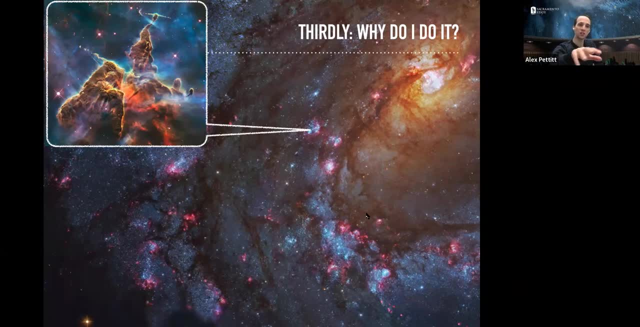 hues showing where the young stars are being formed, and the darkish bands here are dense collections of dust, like little solid particles that are very good at blocking out light. So these big clouds are humongous structures, millions of miles across in their size, And within them is where stars are formed. 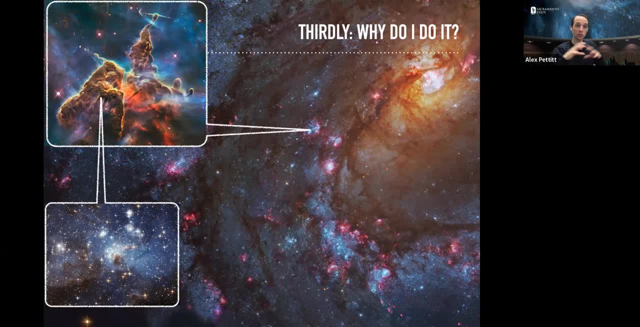 So these giant clouds of gas are the birthplace to young stars, clusters of very young stars, So the brighter, bluer regions in this picture is the gas being ionized, so being stripped of its electrons by the radiation from these young stars. 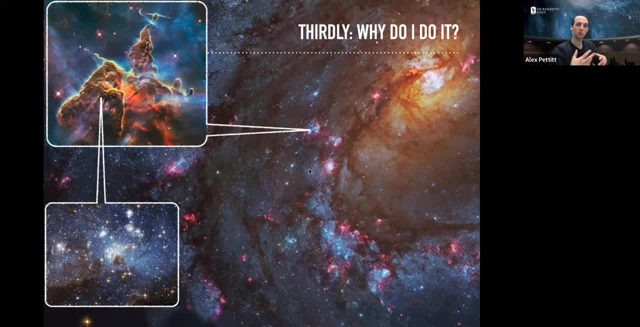 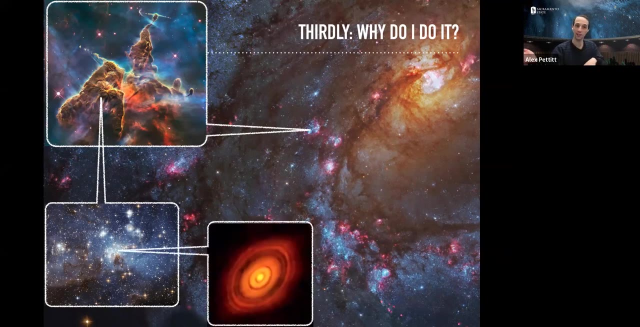 So these young stars spit out a lot of heat and light and that interacts with the gas and illuminates it in these beautiful colors that you see here. And I probably don't need to tell you that it's important to understand how stars are formed, because if we understand how stars are formed, that tells us a little bit about how planets are formed. 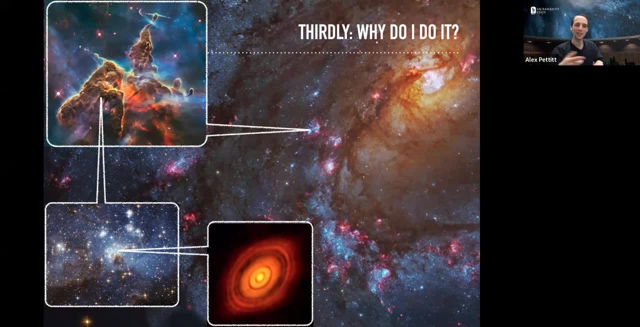 You might have seen this image before. This is a very famous image of a disk of material around a star. So right in the center of this disk, that bright orange, yellowy part, is a young star being formed, and around it is a disk of material that is slowly going to accumulate into planets over the next few million years or so. 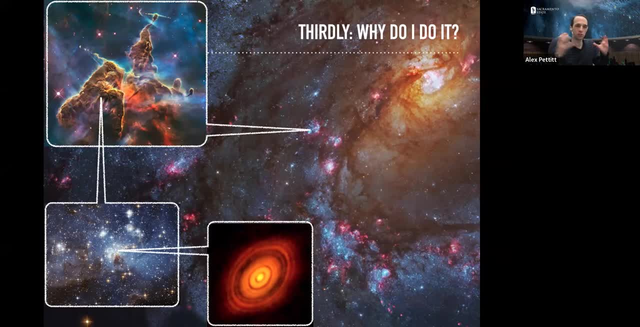 So if we understand how stars are being formed, that tells us a little bit about how planets are going to be formed, which is obviously important because, as humans, we want to know what makes a planet right, What determines the properties of planets. 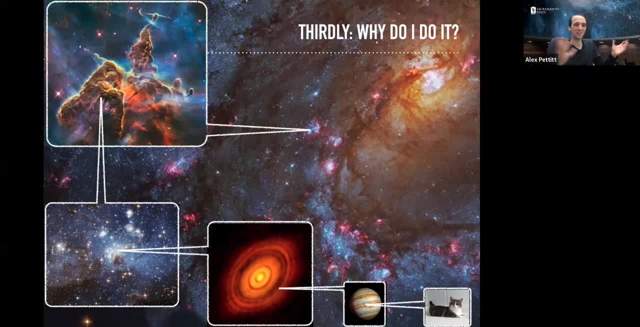 Because ultimately this tells us about life. right, We know the conditions on planets, We know a little bit about the life that is found upon those planets. There's kind of like a ladder here. If we understand how a galaxy forms, that tells us how it builds up its big collections of gas. If we know how it builds up its gas, we'll know about how that gas will form stars. 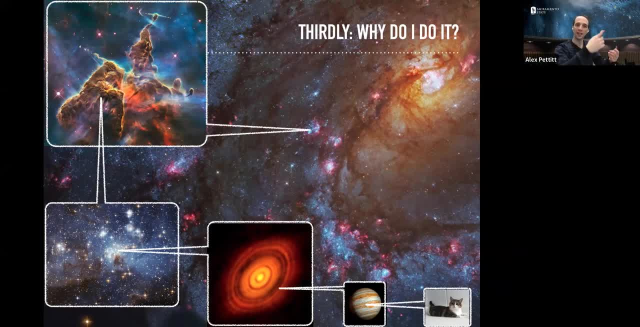 Those stars will tell you about the kind of planets they'll form around them, and those planets will obviously be very important for us. as humans. We like to know about the properties of planets and whether they could host life or not. So it's a bit of a justification as to why it's important to understand galaxies, because it all feeds down the conditions. the large scale determines what's going on, smaller and smaller down as you get to. 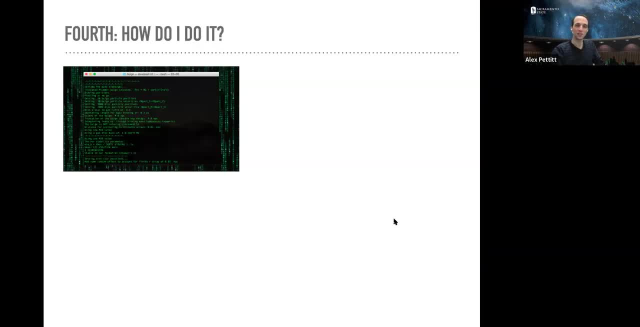 tinier and tinier sizes, So. so how do I do it? So I can't go and stare at a telescope for billions and billions of years to see it change. Galaxies are so big and so all you'll have to watch them for hundreds of millions of years to see them change. They just, they're just too colossal and too far away. 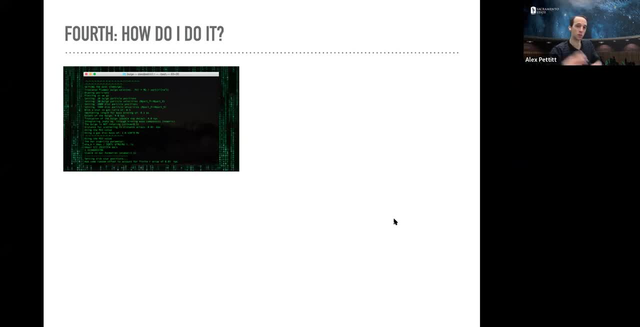 to see a big difference. that's why we use computers, because we can make a kind of a toy version of it, put inside a computer and study it. so i spend a lot of my time writing and analyzing code that replicates how that galaxy should behave. that code is then sent off to a very 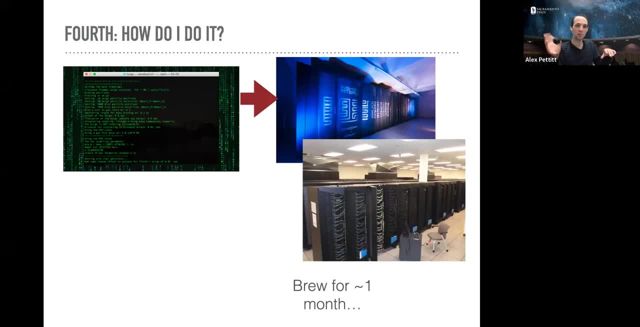 expensive computer in a bunker somewhere. so i use supercomputers in japan and america and canada and england. huge collections of tens of thousands of cpus that we have to apply for, time for and justify the use. send it there. cross your fingers that you don't get anything wrong. 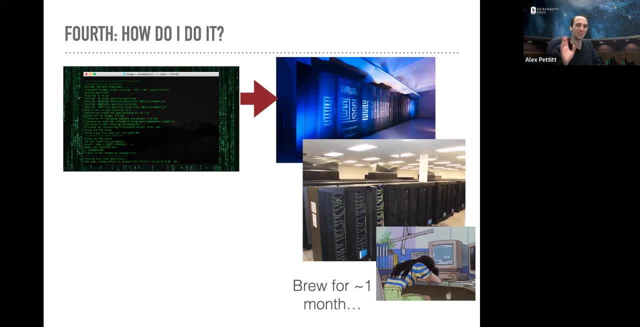 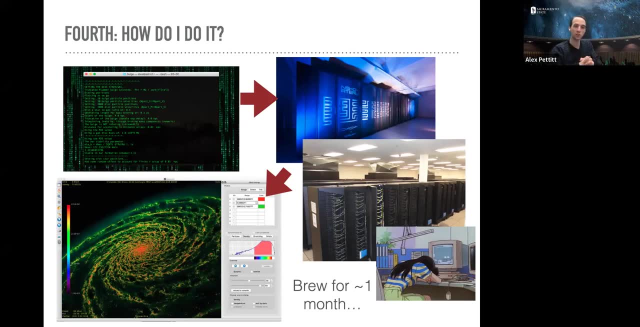 wait for a month or so to hope that it all comes out right. the other end, i didn't get a zero and a one mixed up somewhere, and at the end of it i should hopefully have a galaxy fit enough to do research on that. it's there to answer some problem i've posed when i suck up this simulation. so i've 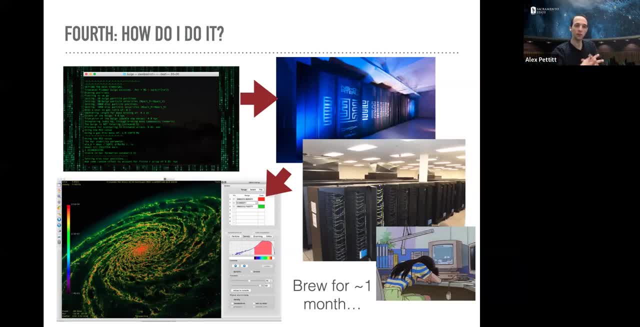 had some idea, put the galaxy together and let it evolve for a few hundreds, millions of years- which takes an order of a month or so- and then study it out the other end. so when i do this, what do i have to consider? i don't just like cross my eyes and put some random. 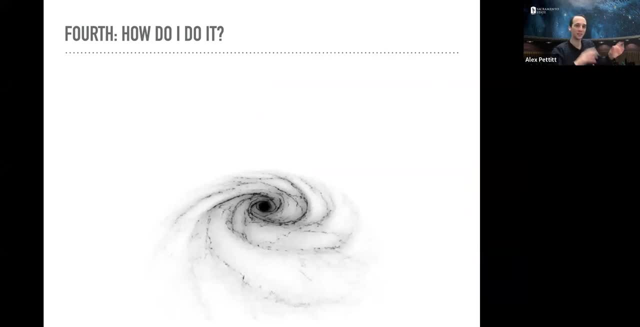 numbers in, i have to think a little bit carefully about the physics involved, right? so i've got to take my time here. otherwise, as a phrase in computers there's garbage in and garbage out, right? if i set up the condition badly, you're going to have to think a little bit more carefully about the physics involved. 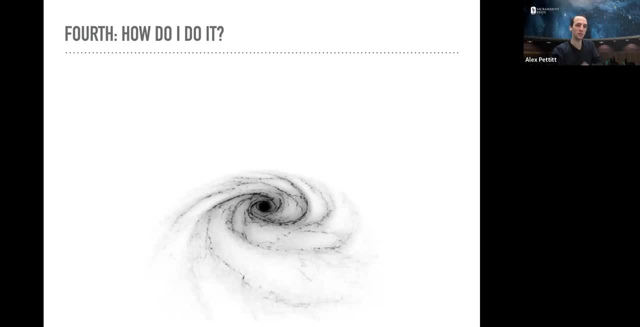 i'm going to get rubbish out the other side. so you have to be very careful about how you perform these simulations. first and foremost, you don't have a galaxy without gravity, right the simplest thing: it has to gravitate. if it doesn't, stars are all going to fly out and it's not going to. 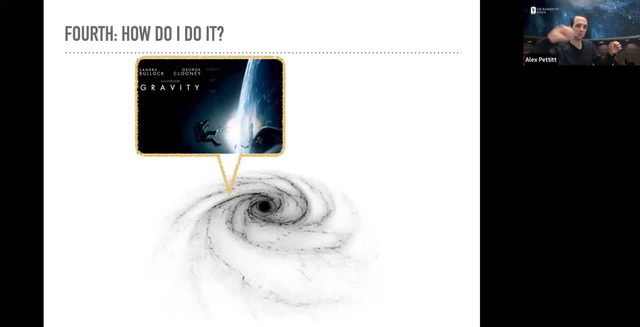 behave as you expect it to. so the simple thing: it has to be able to gravitationally attract itself. but remember i said there's a lot of gas inside these galaxies. right, there's about 10 percent of their mass and this is what forms your star. 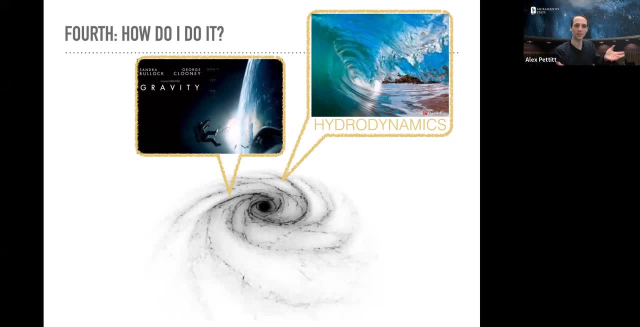 well, gas is basically a fluid. it's just a very thin fluid. so i model the gas using hydrodynamics. the hydro there is means like a fluid. dynamics is how it moves. so there are equations of hydrodynamics in there that govern how the fluid of the gas should behave. so it's a response to 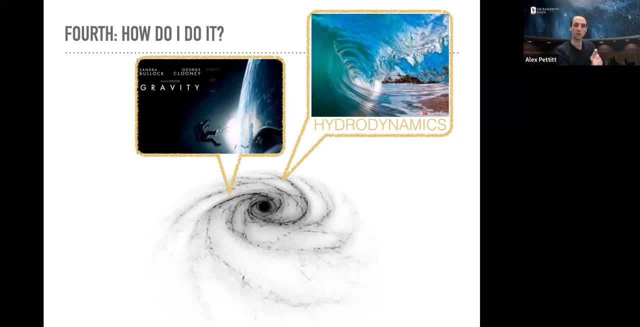 its pressure and its temperature. what is its density going to be? where is it going to move? that kind of thing. it's very different to solid particles if you think about it like one dot on another dot will interact via gravity, but a fluid will distort and compress and change its density. you've got to. 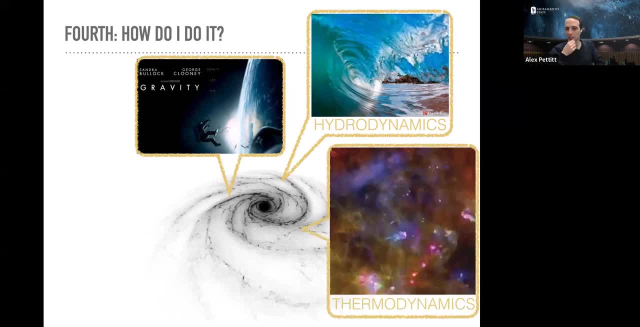 take these sorts of things into account. but then you need a way to get the temperature of the gas right, because there's a lot of processes going on out there in space that alter the temperature of the gas. it's not all about two degrees kelvin, which is sort of the temperature of space. it changes in temperature depending on. 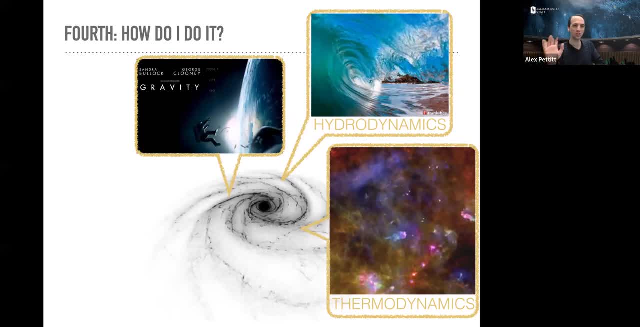 how much gas you have, due to a whole host of reasons that i'm not going to go into here, but But suffice it to say you need to be able to model the kind of temperatures you expect in different regions of space. For example, you have gas around a very young star That's going to heat up that gas really well. 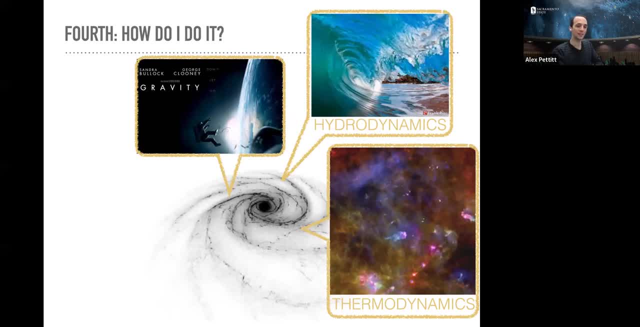 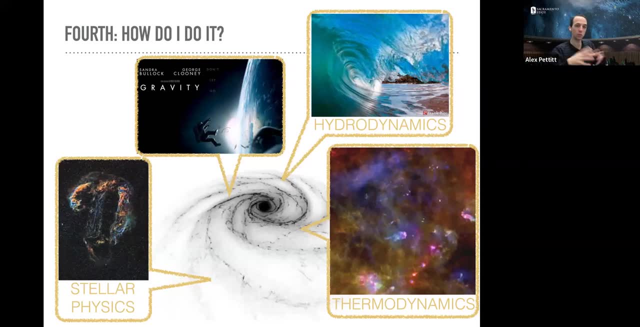 So you're going to have to take care of that effect somehow. And lastly, you need to actually be able to model these stars as they form. So the gas will be forming stars over time. Well, when should it form stars? How many should it form? 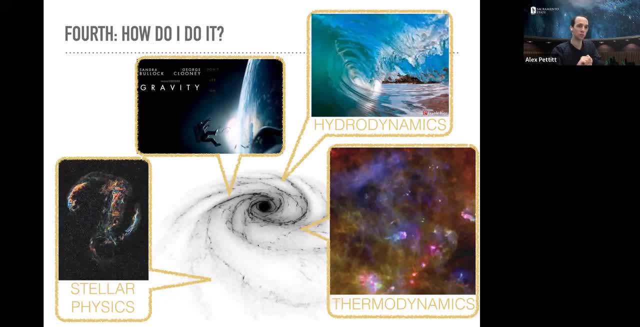 How long will those stars live for? Will some of them eventually go supernova? I think everyone might have heard of a supernova before right- Giant, colossal explosions in interstellar space. When that happens, it's going to affect your galaxy, So you need to incorporate that kind of effect: a big explosion basically going on. 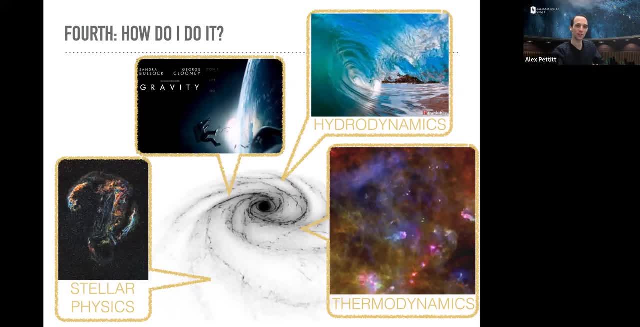 How do you model how the energy is going to move as a result of something like that? This is a broad idea of the kind of things we have to take care of. There's some other things in here as well, But these are kind of the four of the most important ones you need to take care of when you do this sort of thing. 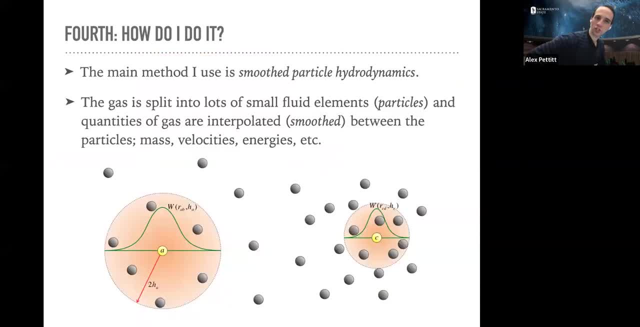 So when I was to give this talk, I was asked to give a little bit of an overview of the method. So I've got a couple of technical slides here about how I actually do this simulation And I think some people might find it interesting. If not, don't worry. In a few seconds I'll go back to pretty pictures. 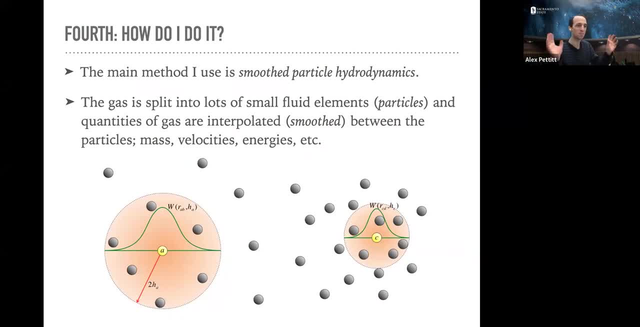 But I do this whole thing of simulating what a galaxy is in a method called smooth particle hydrodynamics. So break that apart for a second Hydrodynamics. I've already told you what that is. That's the fluid moving around. 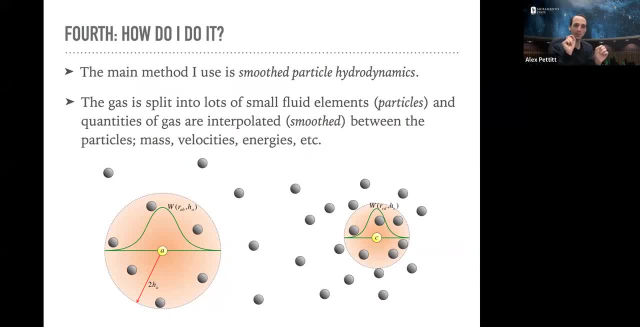 Particle means I Break the fluid up into lots of different little bits. So this picture down the bottom here these gray dots represent little packets of fluid. But we know that fluid isn't really dots separated this amount. There's some forces to it. 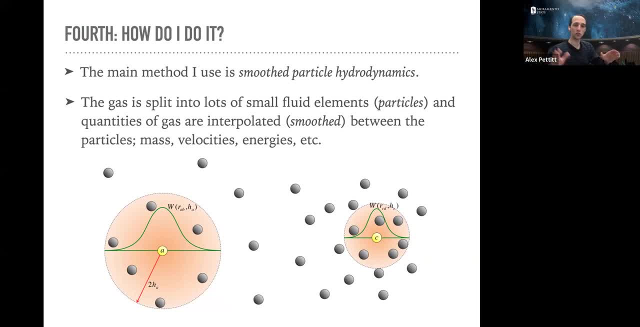 Some of it is bonded together, So the smooth part refers to their properties are sort of smoothed across to their neighbors in a bell curve kind of fashion. So you take the properties of these particles- the yellow ones in this picture at the bottom, for example, and you smooth their properties across. 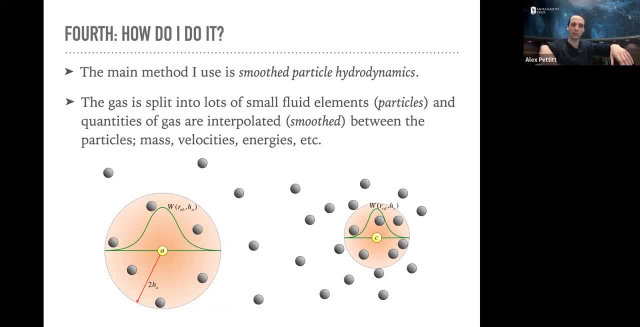 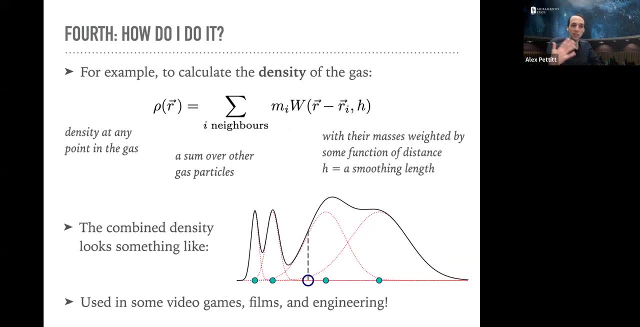 And you sort of take an average, in a sense, of all the particles around and that's essentially, in a nutshell, what the method is. to give you a little bit of an example of how something is actually calculated, Say, I want the density of my fluid. 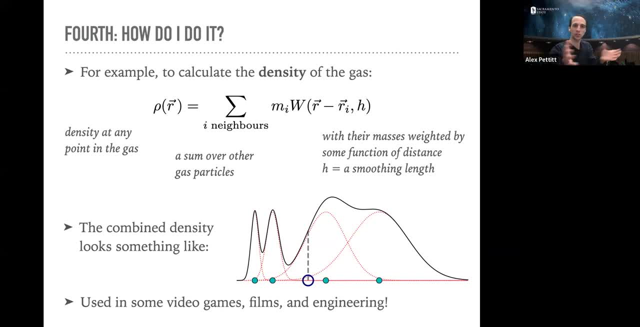 So row of some position are on the left. So the density in your fluid- somewhere you would find this out by adding up that big sum- is addition. right of all the little masses, the end there of the neighboring particles With some. 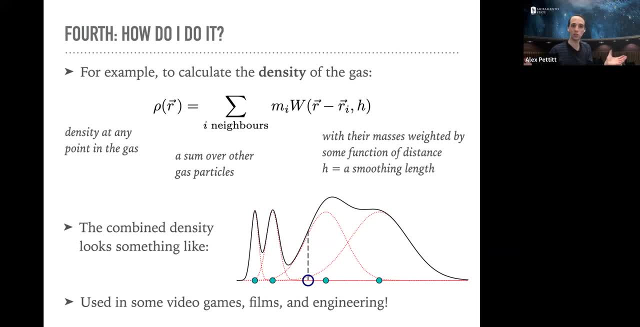 Kind of waiting. So some maybe Gaussian waiting to its neighbors. that big W is what that means. So in this picture down the bottom maybe I want the density of that blue circle To get that I would take the masses of all those green particles and smooth them across and add all their contribution up where that blue circle is. 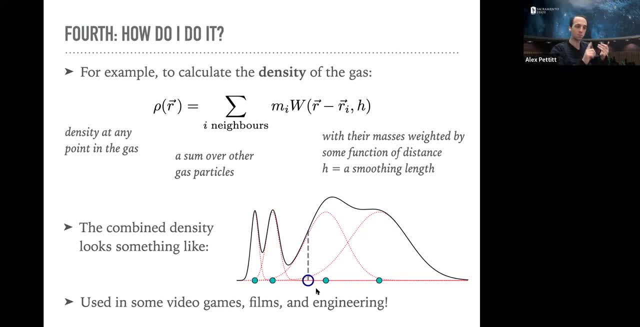 And in a sense that's how the method works. And you can do this for other properties, not just density. do it for velocities, energies, all sorts of properties. You take this sort of Average with smooth things out and a kind of fluid like fashion. 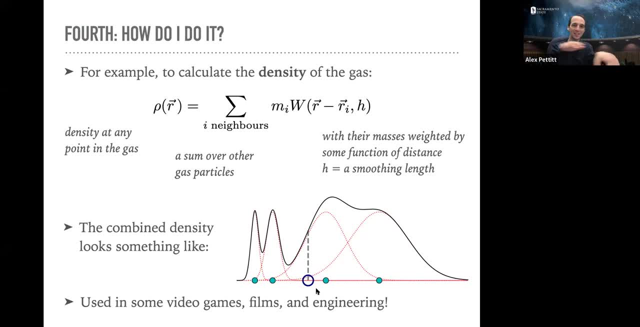 And as the particles move around, these densities are going to change. So it's a. it's a very, very quick and very efficient way to do this sort of problem, And it's used in films, and engineering applications use this sort of thing a lot. 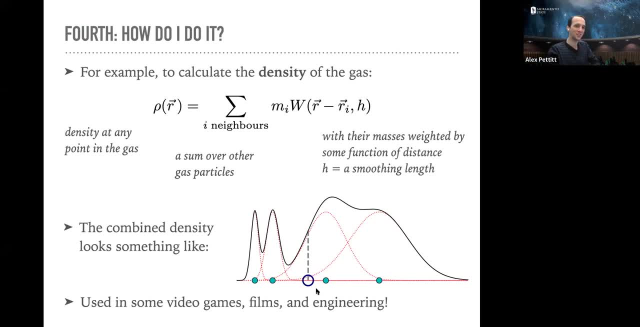 And it's now at the stage where video games are just about starting to use this sort of technology. It's usually a bit too computationally complex, but now that fast enough where they can kind of do this thing for like the body of water. 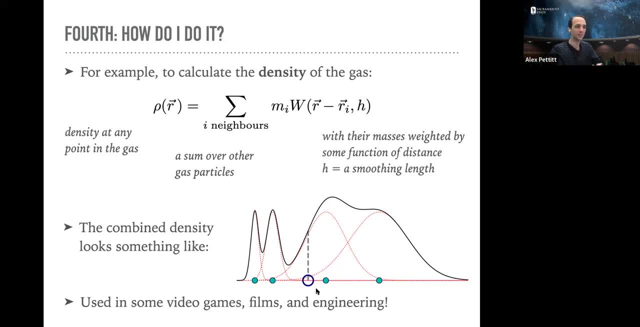 And You know, video game, which I think is pretty cool that they're getting to that kind of speed. So that's how it works. There are other methods, but this is what I, this is what I tend to use, And so now, for the next 30 minutes or so, I'm going to talk through some of the kind of things I'm researching using these methods here. 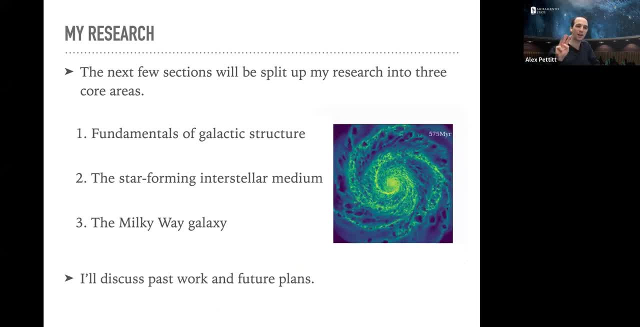 So I've got three, three points of research I'd like to talk about. if I have enough time for the third one, Great. if not, I can put the slides up and you can have a look at them if you're on time. 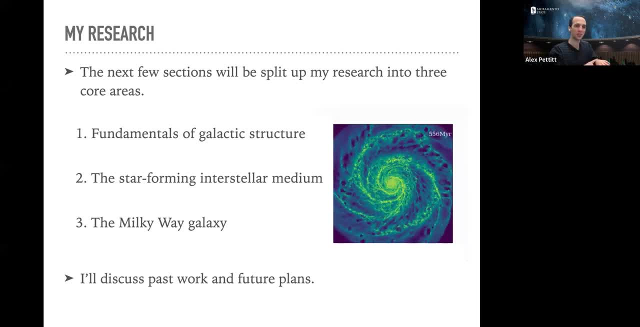 And I do have a little bit Appointment to make in about 40 minutes or so. I have lectures that start up, but we'll see how far we get because I want to leave time for questions as well. So I'll start off by talking about the structure of galaxies in general or the kind of questions that we want to answer here. 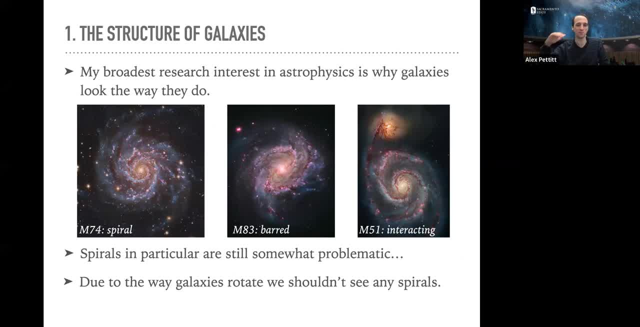 So this is sort of my overarching topic of my research- is why galaxies look like the way they do. So galaxies look very pretty, right. I think that the prettiest things in the universe. you have These beautiful spirals and these long bright bars in the center, and some of them interact with each other as well. 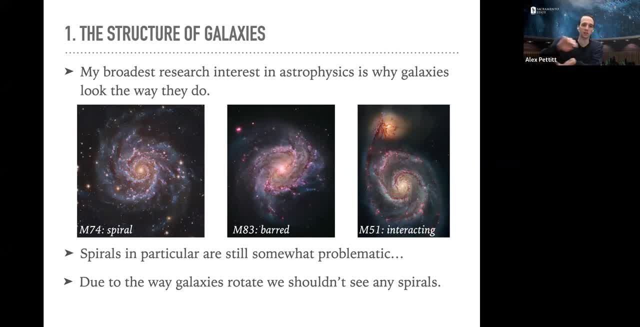 This image on the right hand side is called the Whirlpool Galaxy. It's very famous because it's got these two arms that go up to that bright clump right at the top. That's another galaxy that is interacting with it and distorting it as it goes past. 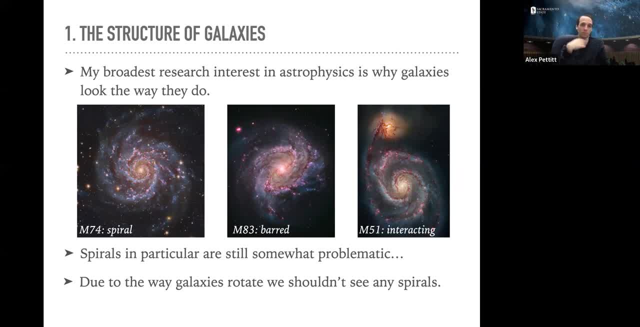 There's a whole host of different shapes and sizes to these things, and a lot of them have these beautiful swirly spirals going around their center, But the problem is we don't really understand why they have those spirals. It's been a topic that's been researched a lot over the past five decades or so, and a lot of ideas have been put forward, but nobody really has the right answers to why they're even there. 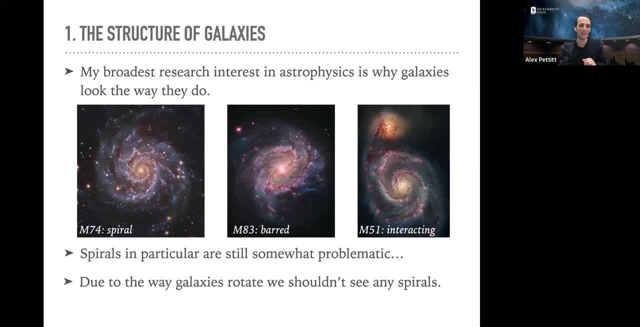 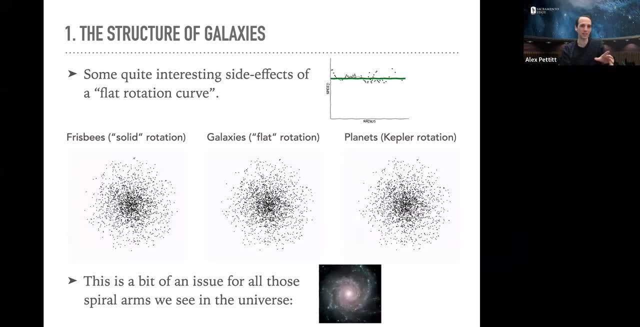 And some of you might have heard of this before if you've taken classes in astronomy. but to illustrate why this is complicated, it's because galaxies don't rotate as we expect them to rotate. So there's something called the rotation curve of a galaxy, which means, if you plot how fast it's spinning as a function of its radius, it doesn't look as you expect it to look. 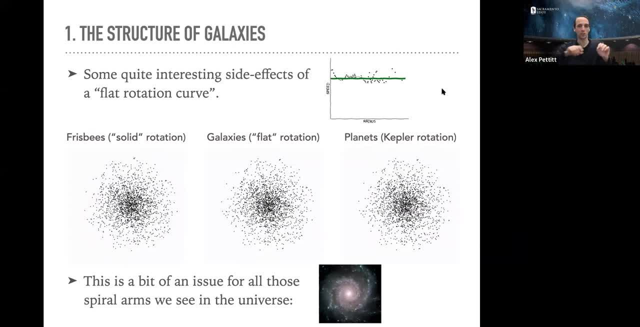 It looks like this little image on the right here, this flat line. So as you move out from the center, the speed stars and gas move around is the same, which is kind of weird. That's not how you expect something to rotate. 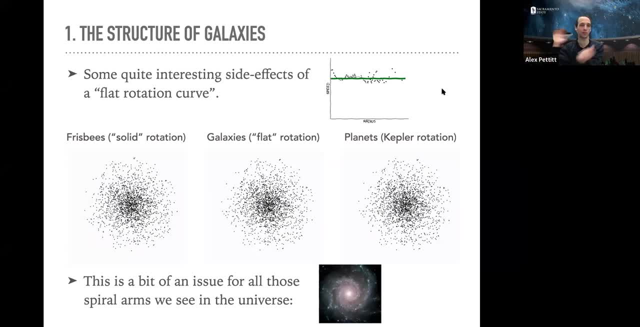 If you have like a Frisbee or some solid playground, That's not how you expect it to rotate. you expect it to go like this: right So, slower in the center, faster at the edge, because it's got more ground to cover. but that's not what galaxies do. 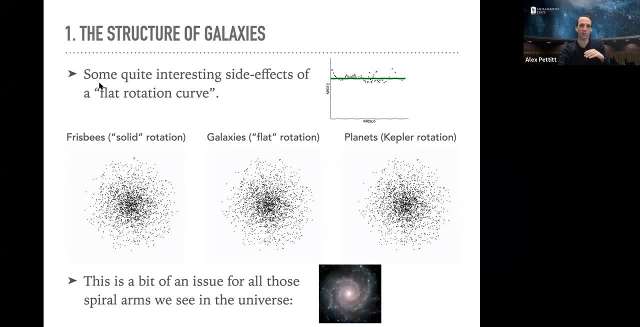 They have this kind of flat line. So to illustrate how this actually looks, these images down the bottom are going to be movies. The left one is like a solid disk, The middle one is a galaxy and the right one is a little bit different. 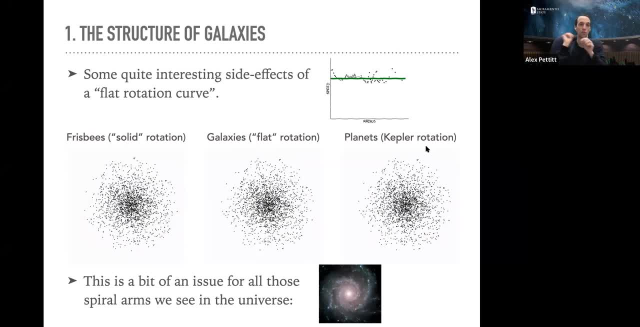 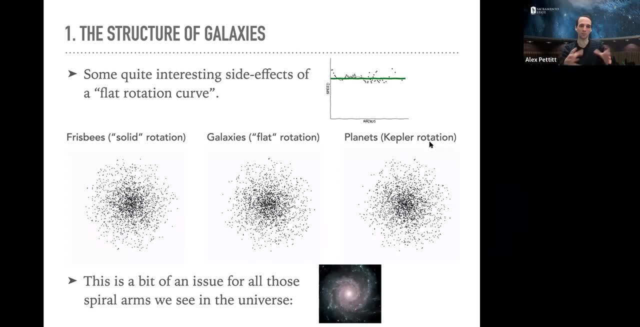 This is how planets orbit. You've maybe heard of Kepler's laws before. Planets go very fast around the center of an orbiting center of mass and very slow Around the edges. So if I animate all of those together, the one on the left is the Frisbee. 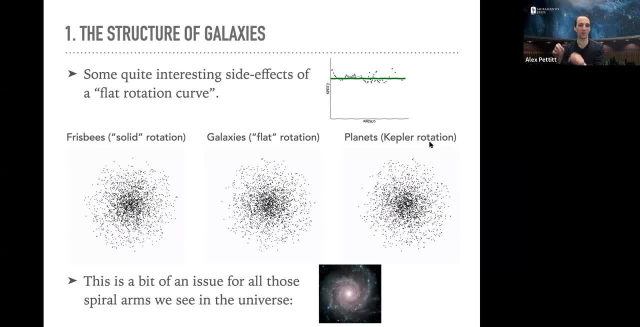 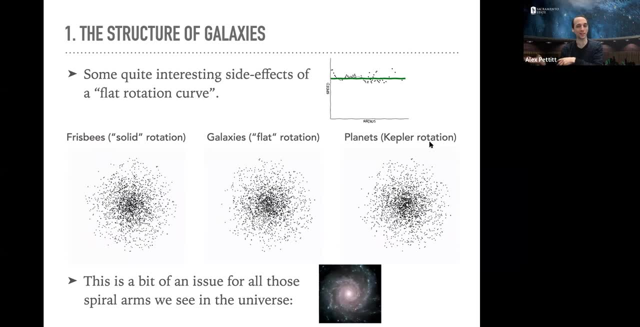 It's just solid, right, It doesn't really change. These are stars moving around. by the way, it's little black dots. The one in the middle is the galaxies, this flat rotation, And the one on the right is how planets orbit around some center. 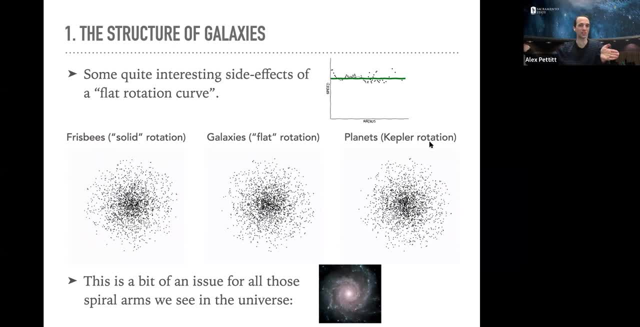 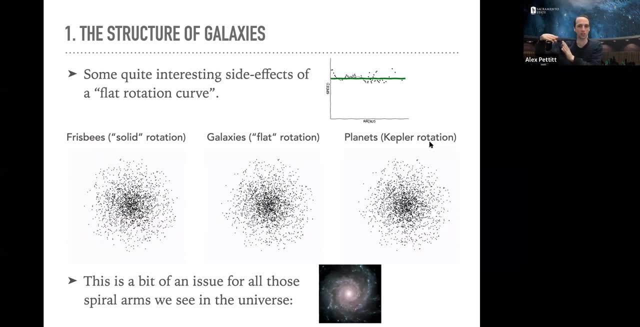 So they're really, really slow at the edges because of something called Kepler's laws. In the center they're super fast, But galaxies have this weird kind of middle ground where they're not really like solid objects and they don't really rotate. 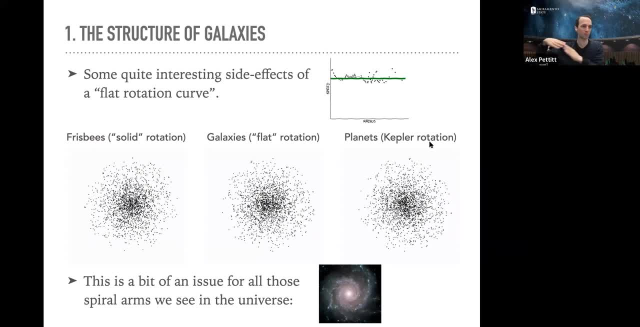 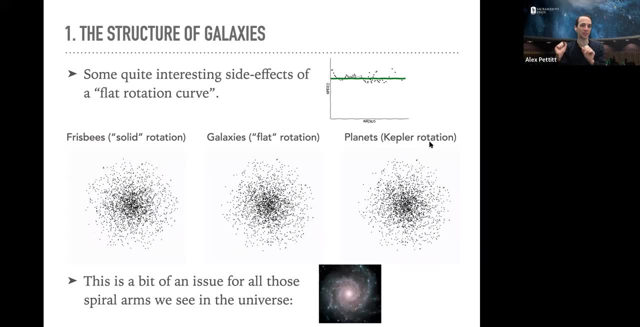 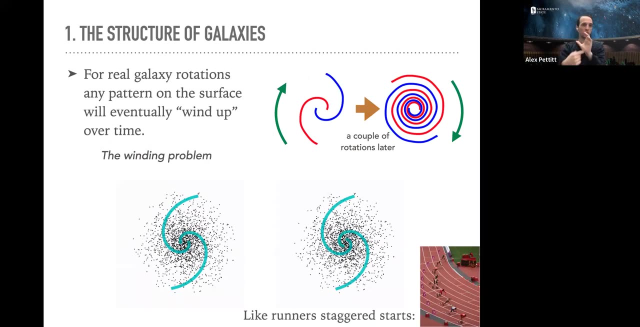 Like planets. quite why they do this is a bit strange. We don't totally understand. We're pretty sure it's got something to do with dark matter. but this is also has problems for spirals on galaxies, Because if they rotate like that, faster in the middle than at the edge, that means any spiral that you draw on it. 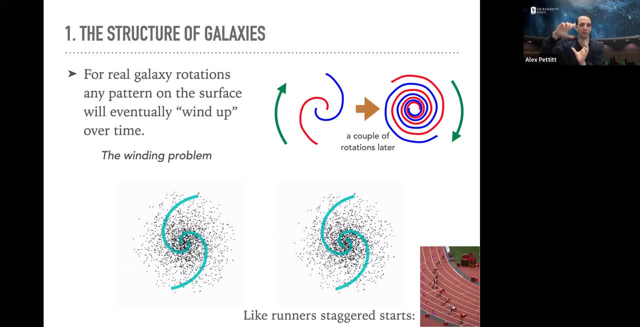 So you take a picture of a galaxy and just draw two spirals on it. if it rotates faster in the middle than the edges, that pattern is going to work. It's going to wind up right If it's not rotating like a solid object. if the middle rotates faster, it's going to wrap around like a tetherball wraps around a post as you hit it. 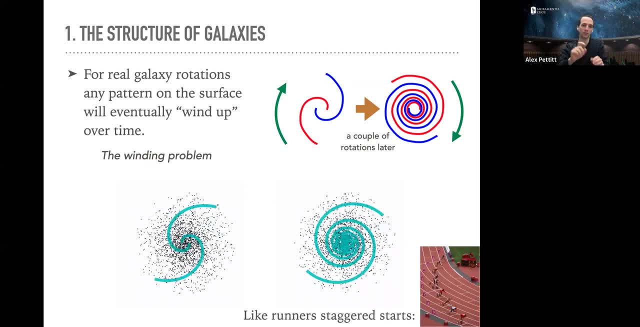 So these little movies on the bottom show you what's happening here. So on the left is like a Frisbee or a disc or a plate. I've drawn spirals around it and it rotates and there's no problem. But on the right is how a galaxy actually rotates. 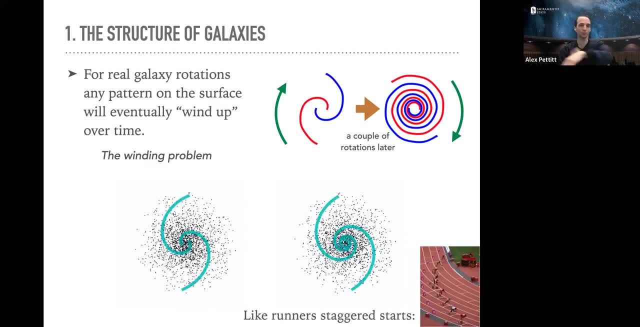 Those spirals wrap around very, very quickly, In the order of like 10, a few seconds, A few tens of millions of years. It's a very quick process. But this is a problem, because we see spirals in all sorts of galaxies very, very frequently. 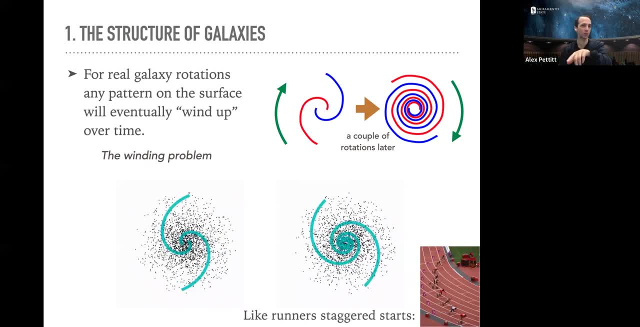 If this is what was really happening, they should all wind up really fast and we would hardly see any spirals around. So something else is going on to maintain these things. There's some mechanism needed to regenerate them, or they're not behaving like we expect them to behave. 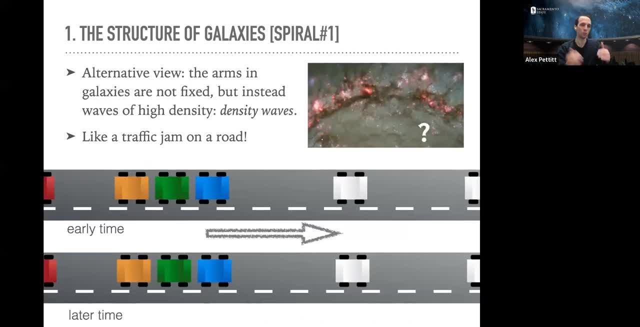 But the historical argument is that we're thinking about these wrong. They're not like fixed things in a galaxy that are always there. They're what we call over densities of stuff, So they're places where there's just a lot of stuff at one given point. 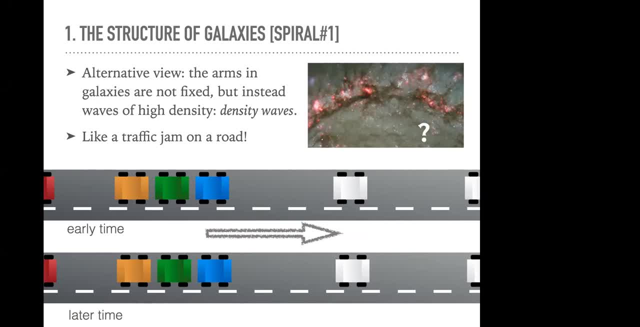 But the stars don't live there the whole time. Stars and gas come through that arm and they leave on the other side, So they can keep this strange rotation And the spiral arms can just move at whatever speed they please like. So, for example, they're very similar to a traffic jam on a road right. 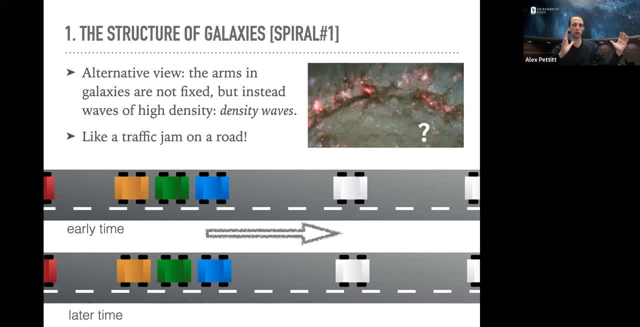 If you know anything about traffic jams, they're just kind of collections of lots of cars. at one instance, Maybe someone braked really really hard one time and they slowed all the traffic down. People tend to move out of the front of traffic jams and come in the back. 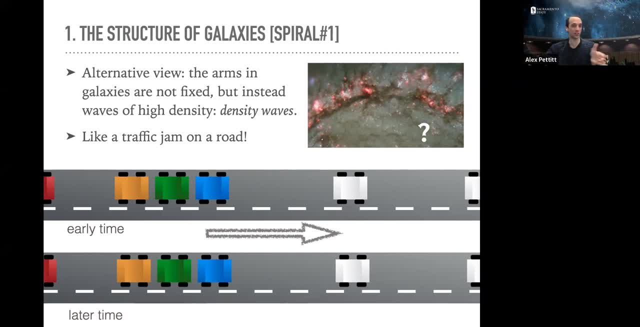 But the jam stays there and moves along very slowly. But cars exit and they enter it. So at the top here is a traffic jam. We've got three cars here. The white one is left and the red one is coming in On the bottom is at a later time. 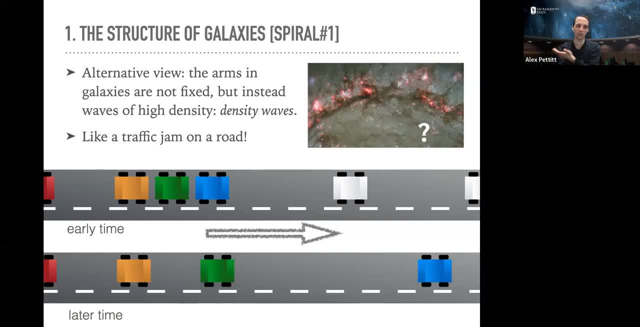 The white cars move along. The blue car will finally exit the traffic, But the yellow and the green one are stuck there still Now. the red one will enter from the back And the white one- another white one- comes along from this side. 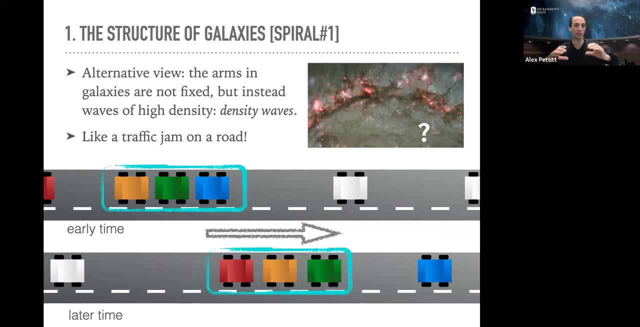 So this collection of cars still marks a place where there's a high density of stuff. right, There's lots of cars at this point, Whereas they've still been allowed to leave. There's still a flow of stuff through this, But it's not the same stuff all the time. 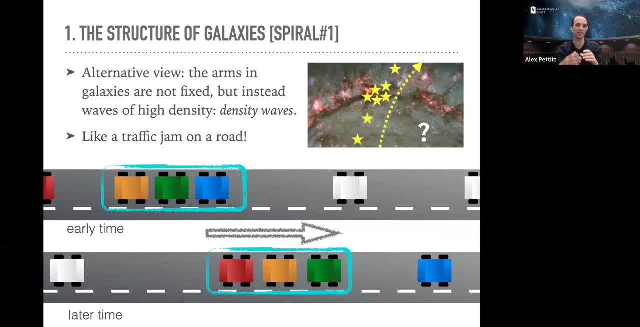 And we think this is one way people try and explain what spirals are. They're just places where lots of stars are spending a lot of time, But they can still flow through, Maybe speed up a bit as they leave And they keep that rotation that we expect the galaxy to have. 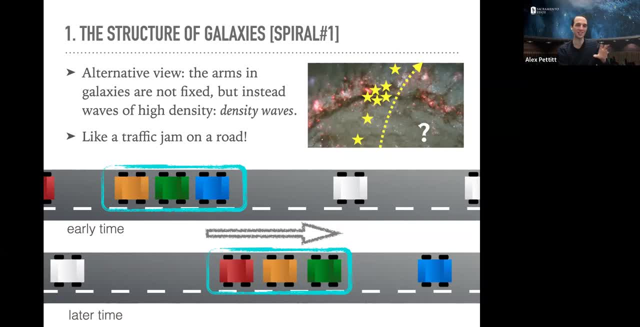 Which is good. This is kind of like the textbook answer to this problem. So if you've studied astrophysics or astronomy in your second or third year, perhaps you may have encountered this before, But it doesn't explain everything. The more we understand about galaxies and the more we look at them through telescopes- 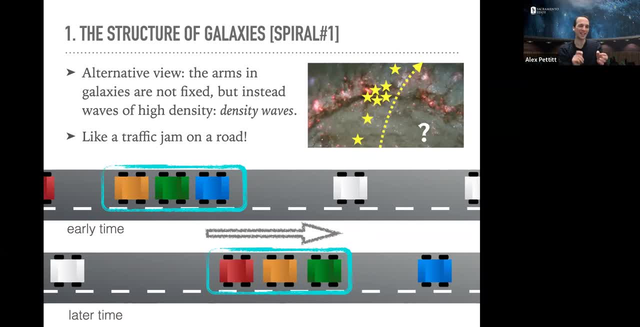 we have ways to test this, to see if it's right or not, And sometimes it doesn't work. Sometimes the galaxy doesn't have the right kind of property, that this is actually what's going on. The speed of the material isn't quite right. 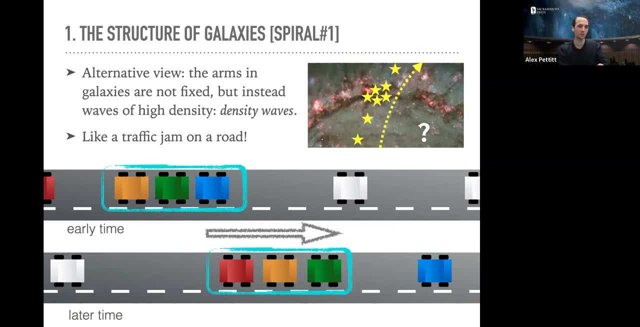 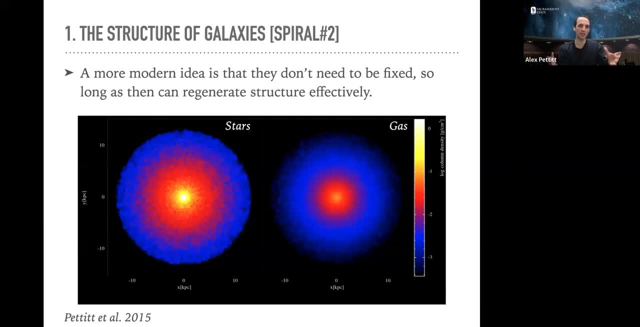 The properties of the arms doesn't agree with what it expected to be. And another thing is simulations can't reproduce this very well. So when we try and set up a galaxy in a computer, making those kind of arms where stuff comes in and goes out, 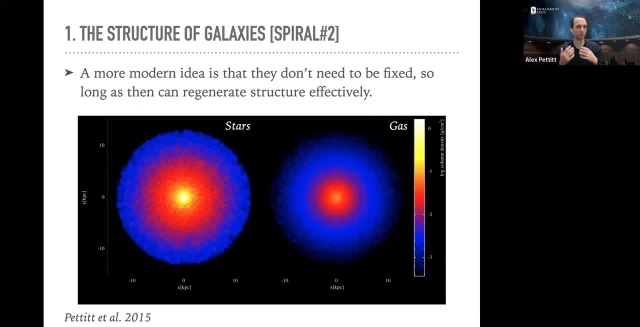 they don't do it very well. We've tried all sorts of different ways of setting them up and different conditions And making them do. that is very, very rare. It hardly ever happens And you have to be very, very particular about how you set it up to make that happen. 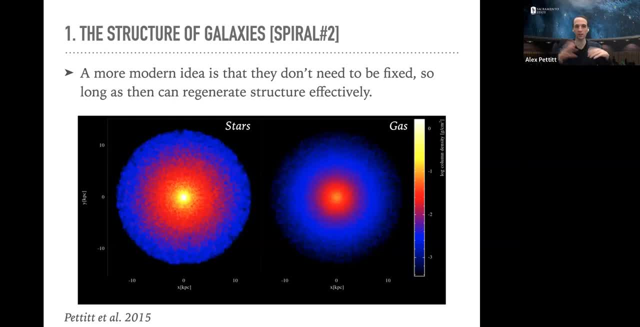 So at the bottom here is a simulation of a galaxy that I've set up. It's two images. It's the same galaxy. I've just split it apart into its stars and its gaps. Normally, when you run this, they're on top of each other. 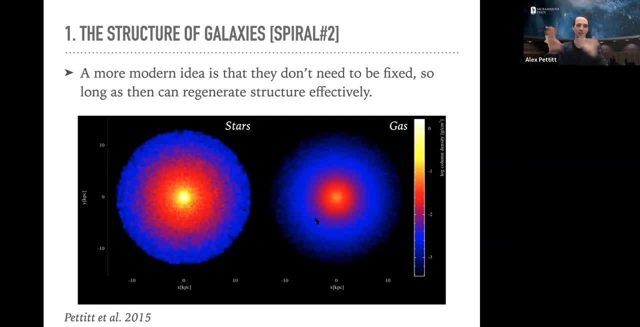 They move and evolve with each other. I've just split them up to make it clear about the different pieces. So if you watch the stuff as it rotates and evolves, you've got. the stars are very smooth, The gas is kind of bitty and filamentary. 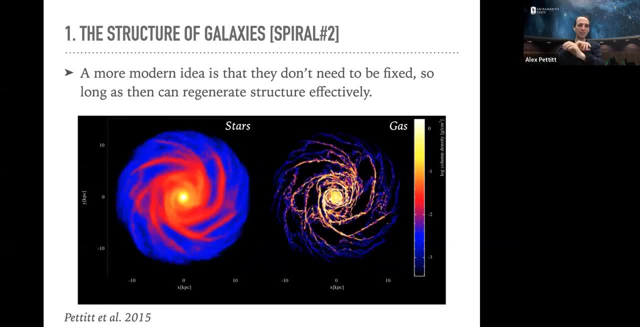 If you look at the arms, they're very dynamic, right. They do wind up and they do dissipate a little bit. I'll play this a couple of times, But they also are formed as well as a very what is sometimes called. 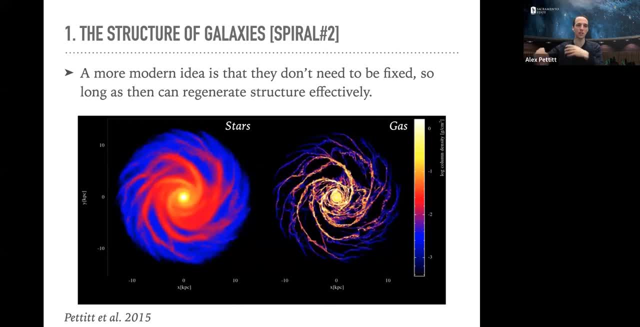 transient or there's a very time dependent nature to them. They come and go on very short time scales, But there's still arms in there a lot of the time. They just come and they go and they come and they go quite regularly on the order of a few tens of millions of years or so. 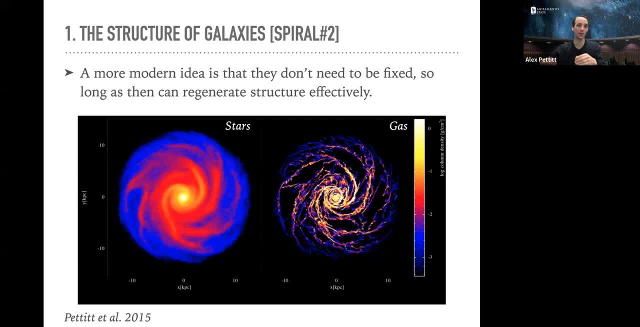 So this is another way you can think about them. They can be just material there the whole time. It's just that they live for very short periods of time and then they're remade again afterwards. The mechanism behind why this happens is extremely complex. 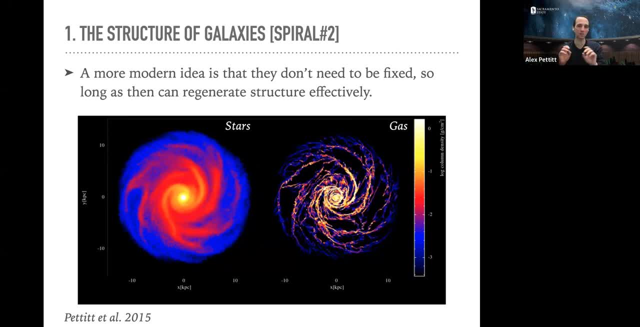 It's complicated to explain, But, in summary, there's some kind of instability in the gravity of the galaxy that makes these features form, And it will keep happening again and again, and again so long as it keeps forming stars. Another very simple way to do this. 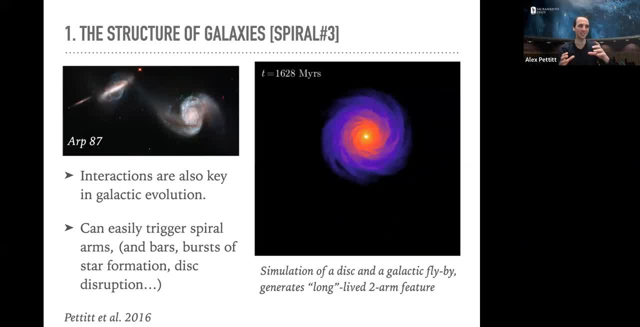 which has been known for quite some time and I showed you an image a second ago- is to interact with the galaxy. So that whirlpool picture before I showed you, with the spiral, with the long streak in the other galaxy, Interacting with the galaxies. 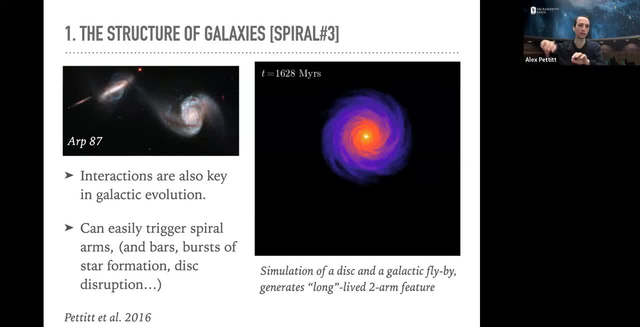 it's a very good way to make arms. So if you heard about tidal forces of the moon on the Earth, it's a similar sort of thing. The companion comes around and the tidal forces distort the galaxy, But because the galaxy isn't a solid object. 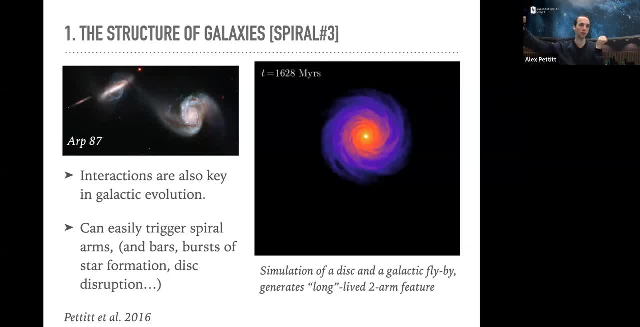 it deforms in a much stronger way and you can pull material apart and it will wrap around and form arms later on. So this image on the right here is a galaxy in the middle and a companion is going to come in from the top And it's gravitational. 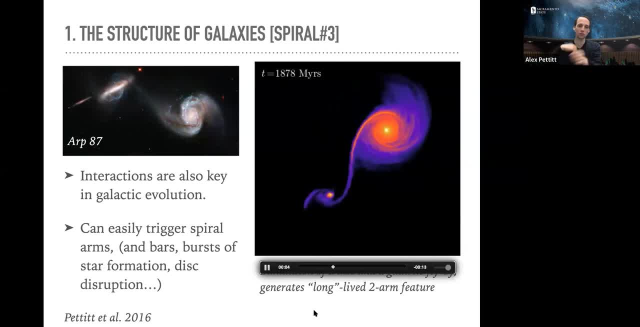 There we go, On the right. There it goes, And its gravitational force distorts the galaxy as it comes past And it generates this beautiful spiral structure And it lasts for quite a long time And it is like a wave, Can you see? 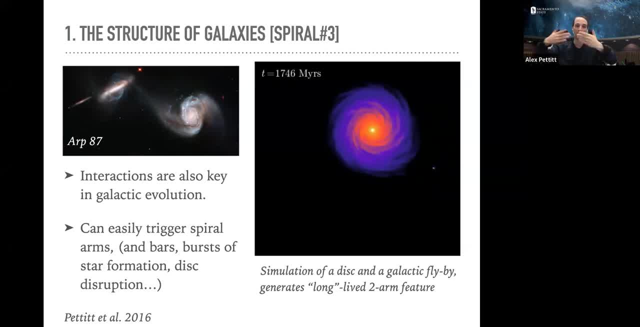 The material is sort of flowing in and out of it. It doesn't look like a fixed structure, It looks like a kind of a wave like you see in water on a beach. Play it one more time. So this is another kind of mechanism. 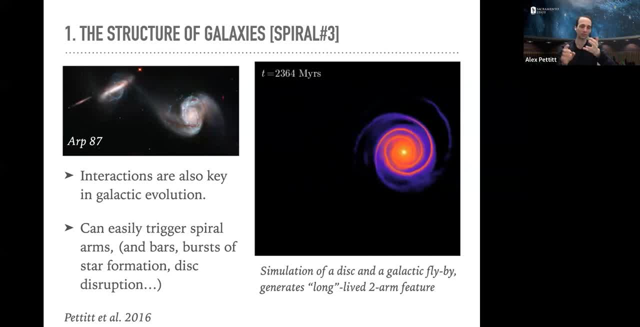 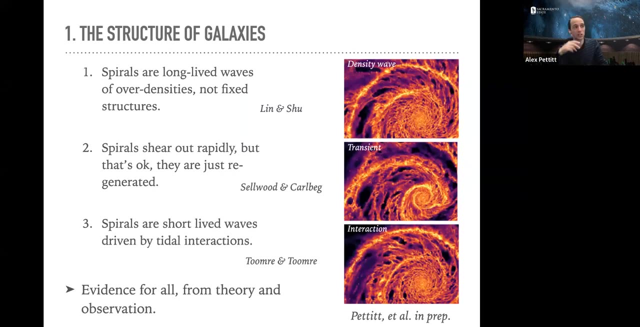 So we can have them as like very steady, regular waves, These transient or these very short-lived arms, or you can maybe generate them via interactions with the galaxies. So in my work- and I'm not going to dig super deep into the details- 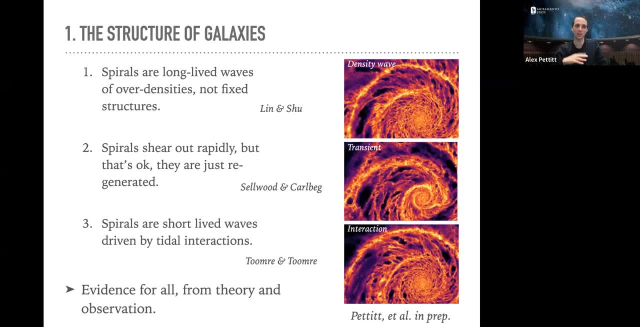 I've done some studies trying to test these different mechanisms of galaxies and how they form arms. So on the right, here are pictures of one you make with one of these steady traffic jam like waves. The second one is one of these more short-lived spirals. 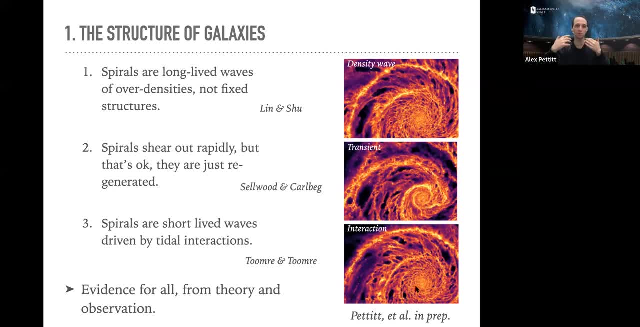 in a galaxy And the bottom one here is something made by an interaction. So some of the work I've done is to make simulations of each of these, set them up in very particular ways. they want to form these three different types of arms and then dissect them basically. 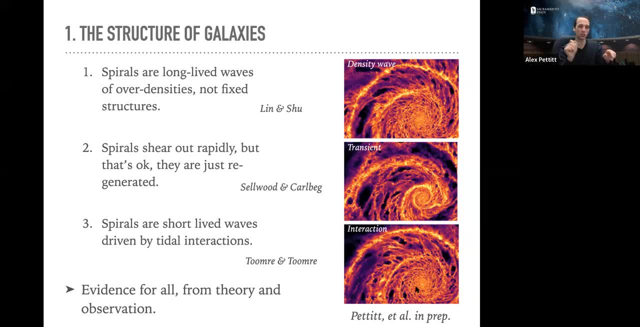 Look at the differences in their velocities, Look at the differences in exactly where they form stars, Look at the differences in how they accumulate their gas, And then compare this to what we've done. Compare this to what we see in real galaxies and telescopes. 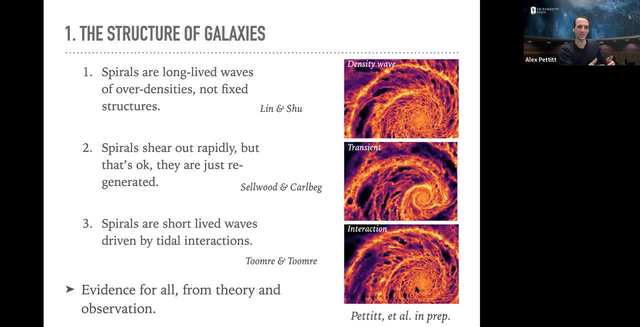 So I didn't put a lot of the results here for this, But what we find is it's actually very hard to try and find a difference, So all of them tend to result in the same sort of features, So they might look slightly different to look at them. 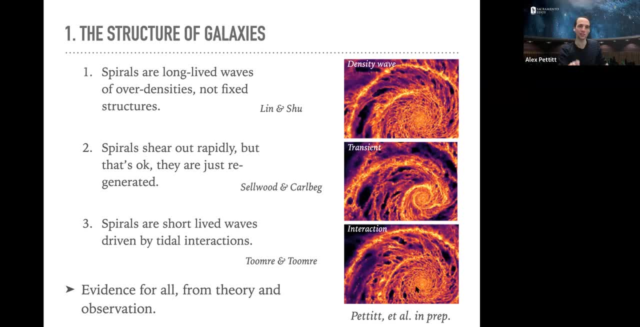 But when you start digging into the details, they're really similar in terms of how many stars they form and how dense the gas gets, And it's very hard to take apart one thing and realize, ah, that galaxy formed an arm like this. 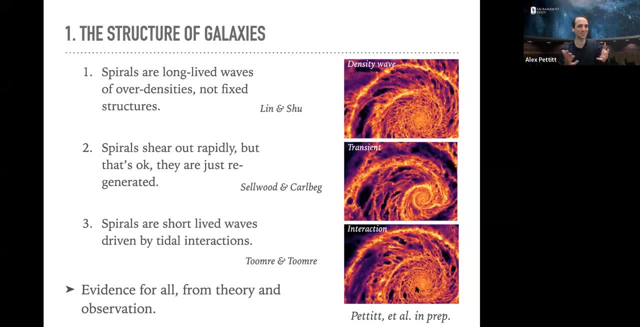 It's very difficult. In a way, it's kind of good news for observers because they don't have to worry about differences, But it means we don't understand it as well. So we're still trying to dig into this, The next thing we're doing at the moment. 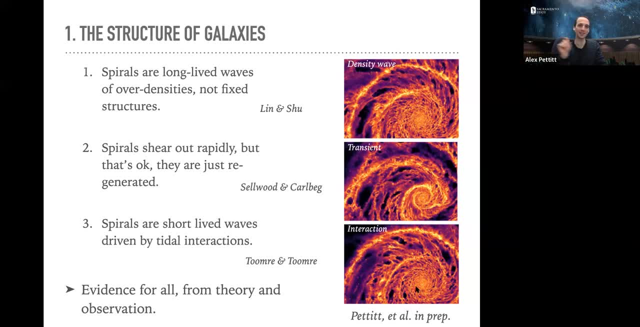 is trying to look at how stars migrate in these galaxies. That's the next thing we're trying. So stars don't always stay at the same radius. They move in and out a little bit, depending on large-scale features. They migrate inwards and outwards. 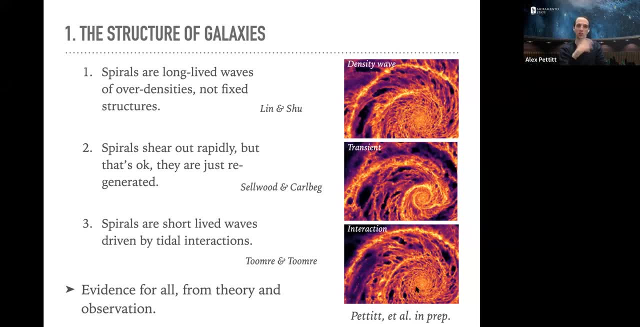 That's the next thing we're going to try and look at. Is there a big difference here? Because there's some measurements of galaxies where we can tell if stars have migrated or not, And that's the next thing we're going to try. 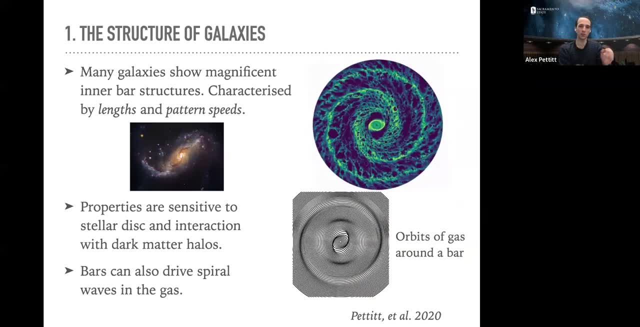 And I also look at other features of galaxies as well. So I talked about the arms, But I've also mentioned the bars right at the beginning, those big, long elongated structures in the center. So there's a beautiful picture here. just a small one. 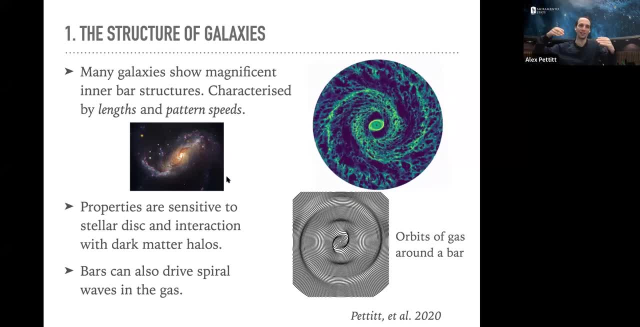 of this bar in the center of a galaxy, this long bright feature here with all the gas running along it. And here's a little movie on the right-hand side of a bar in a galaxy. I made the movie so that the bar doesn't move. 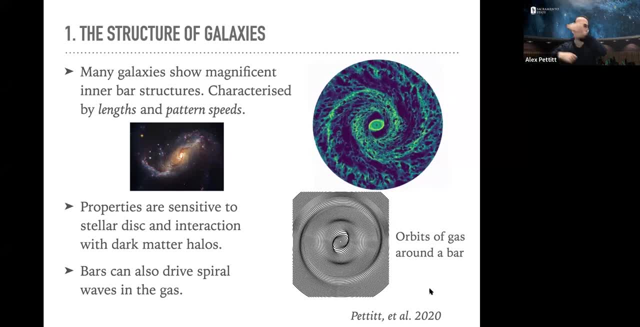 The bar is always angled top-down And you can see all the gas around it, as it behaves and feels the presence of the bar And it drives it into these sweeping tails coming off from the top and the bottom of the bar. So I study these a little bit as well. 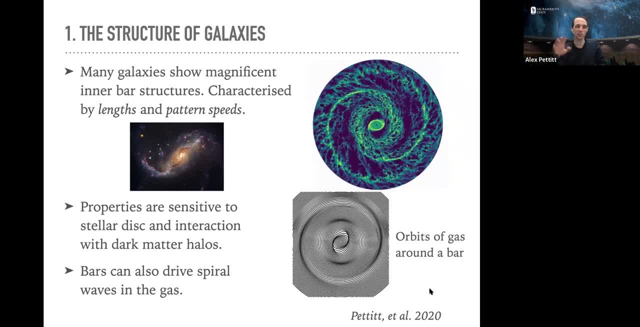 And some of the recent work I've done looking at these has been to study how they behave if the galaxy is interacted with. So I talked about interactions already before. I kind of like interactions of galaxies. I think they're really cool. They make some beautiful images. 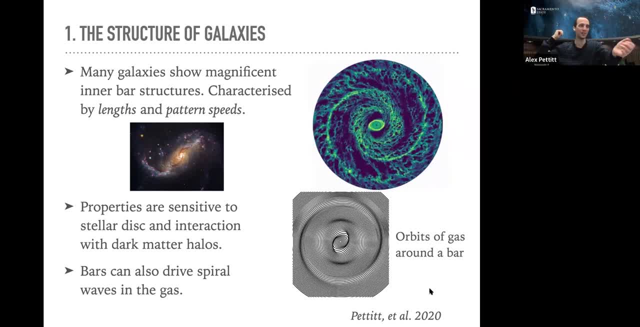 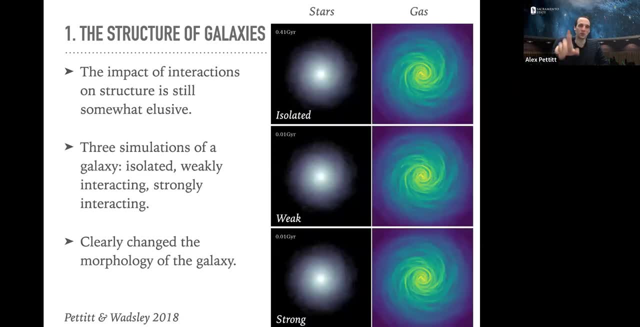 and some of the craziest things in astronomy when they eat each other up and what we call cannibalize two galaxies together, as they really destroy each other's structure. So here are some movies of a galaxy that wants to form a bar and how that bar changes depending on if the galaxy 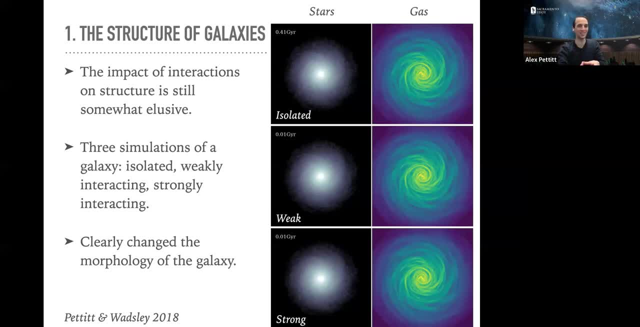 is nice and lonely in space, if it's just on its own, if it's been interacted with by a small galaxy, or it's been interacted with by a large galaxy. So each of these kind of events might distort how it evolves and how it's going to form that bar. 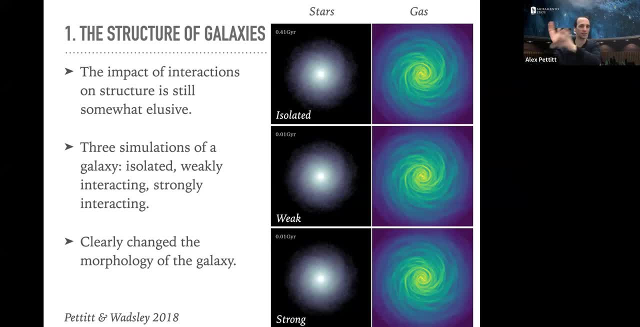 And I've shown them in a similar sense to before. So the stars are on the left, The gas is on the right In reality. remember, these are simulated exactly the same time. I've just made pictures of each one separately so they're easy to look at. 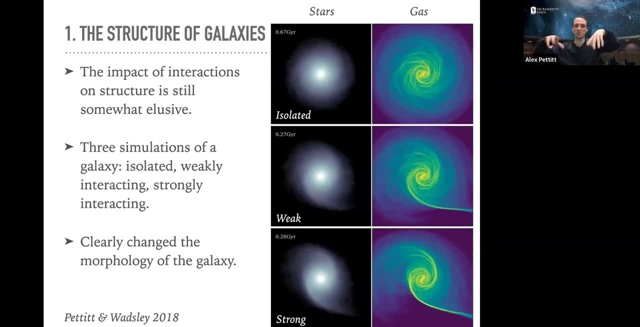 Well, I do them all at once, So the isolated one maybe take a second to look at one and I'll play it a few times. So the middle one and the bottom one have been interacted with and it triggers different kinds of structures in each case. 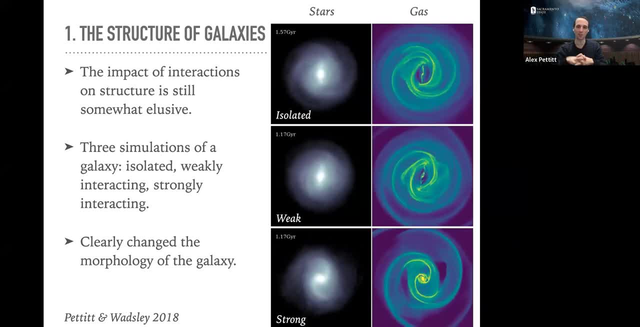 The outskirts in particular are much more dynamic, And the one at the top is just forming on its own. So you can see some differences in each case. There's a point here where the companion is very massive. It does make a big difference. 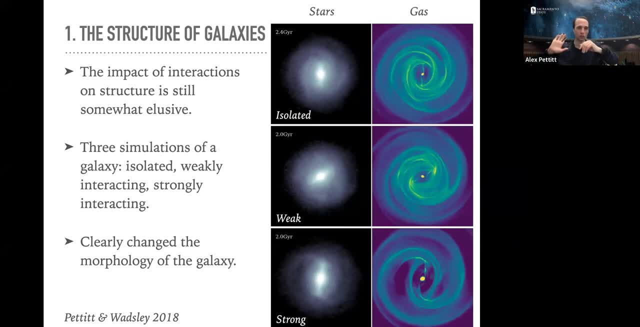 But for the middle one and the top one, giving it a little shunt with a companion didn't do a huge amount. It changed a little bit but it didn't make a huge difference. I'll do that once more. You just about see the companion go off to the right-hand side. 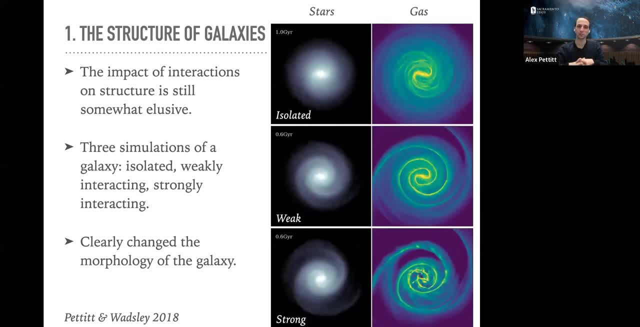 as it comes and sweeps past. So even with the ones that have just been interacted lightly, the end result is very similar. It rotates about the same speed, It has roughly the same properties, It's the same size, But the one at the bottom has been interacted with strongly enough. 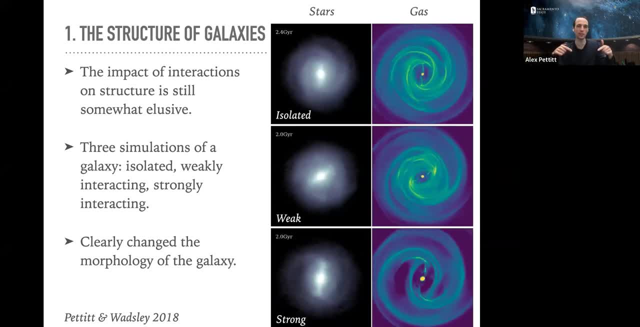 It's distorted the galaxy and has funneled more material into the center, which has helped build a much bigger bar than the other two, And I do the opposite of this kind of stuff as well, So I also look at a galaxy that doesn't want to form a bar. 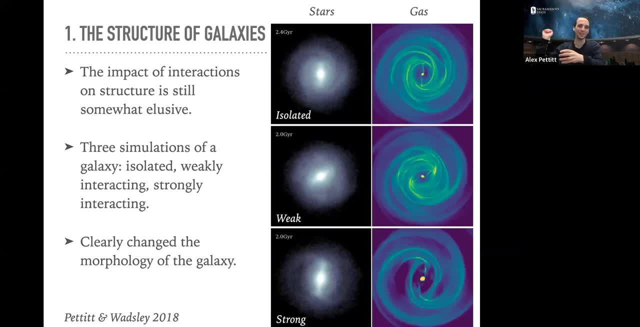 Can you make it form one if you interact with it, And then sometimes you can If you hit it heavy enough. basically it will be stabilized and form a bar at the center. I've talked to you about very general galaxy things so far. 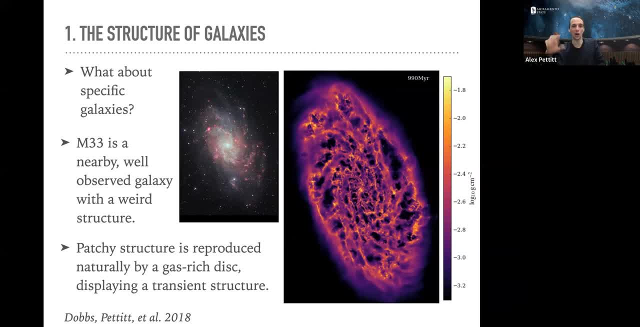 like: what arms are, what bars are like. I also spend some time looking at specific galaxies as well, So this one here is a very famous galaxy called Triangulum- this beautiful image in the center, or M33.. It's quite close to us. 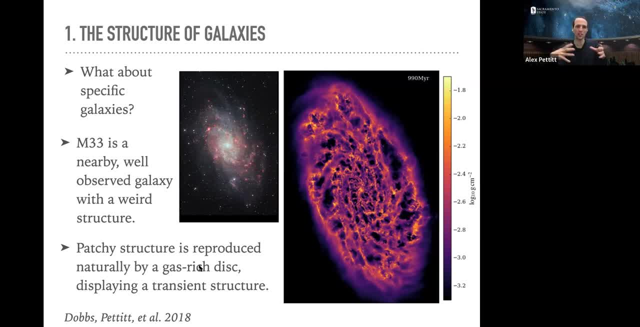 It's a bit small. It's about 70% of the size of the Milky Way, but it's still a disk galaxy. But it has this very not defined structure right. When you look at it it's kind of got some arms and there's some bright patches. 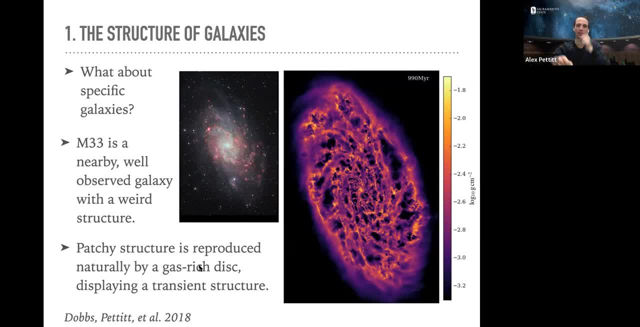 but it's not as clear as the other pictures I've showed you, which are very nice, sweeping spirals from the center, So it's a bit harder to tell what's going on here. So some collaborators and I set out to try and simulate this thing. 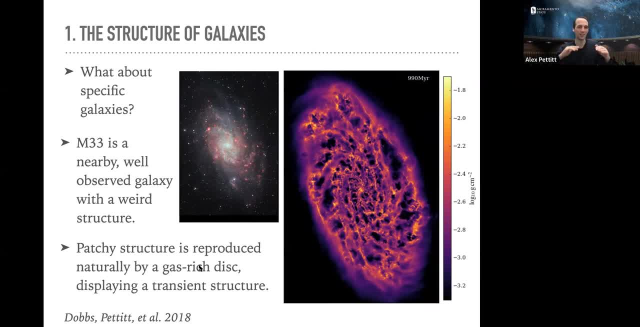 and understand why it looks like the way it does. We carefully reproduce how much gas it has, how much stars it has, how much dark matter it has, and see if we can match the properties. This thing on the right is a movie of one of the best simulations. 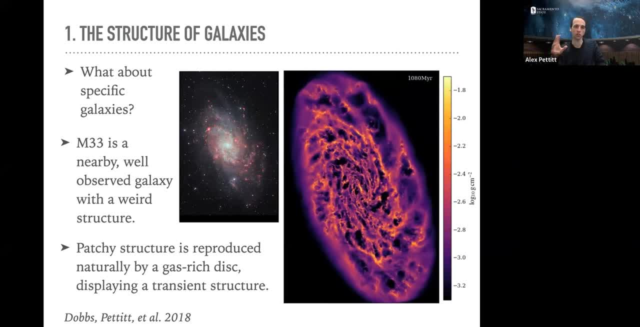 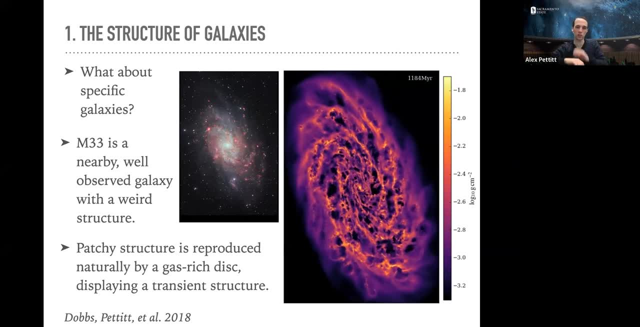 that we made. that reproduces what it's doing. This movie is just the gas. I don't have one of the stars, I'm afraid, And later on as it evolves a little bit more, you can see we generate these kind of bitty and not very clean spirals. 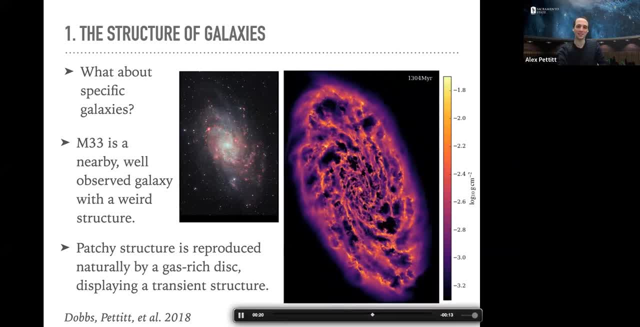 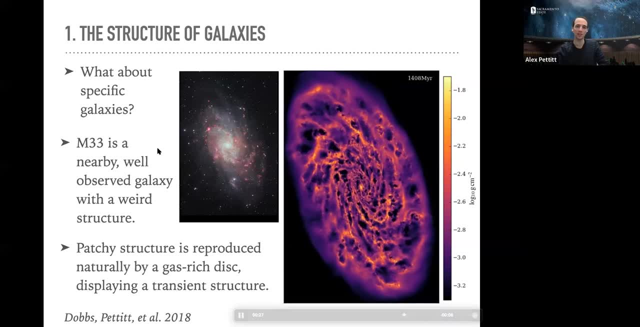 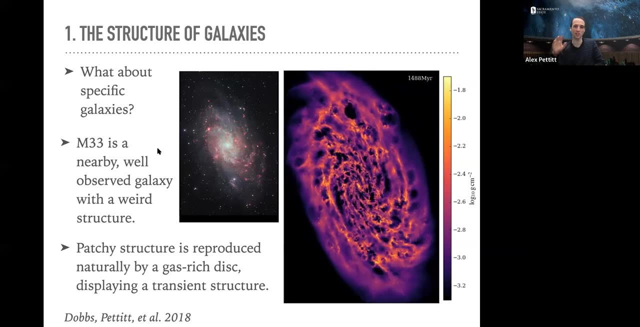 that match the structure decently enough. So you can see that there are still little spiral segments in there, but they're quite small and they have a good overall match with the kind of spiral bitty filamentary features of the real galaxy. But what's interesting in this disk is that all these features here 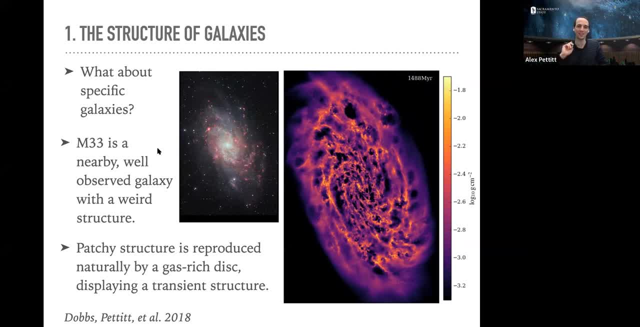 are basically driven by how well the galaxy is forming stars. So you see, there's lots of like gaps in the galaxy. There's lots of big holes and cavities. These are driven by pockets where lots of supernovae have gone off At the same time. 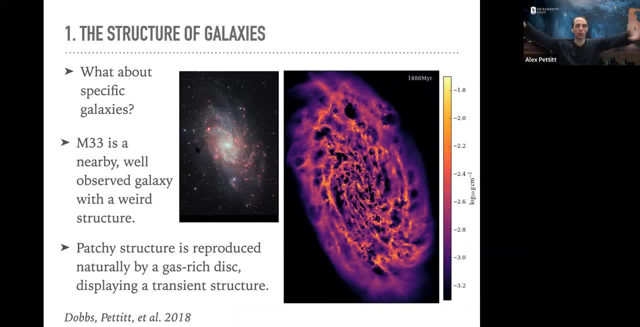 So they've made lots of young stars and they've got very massive and have blown out lots of this gas And that has repercussions for the galaxy because it has so much gas in it that determines how the gravity at that position is going to change. 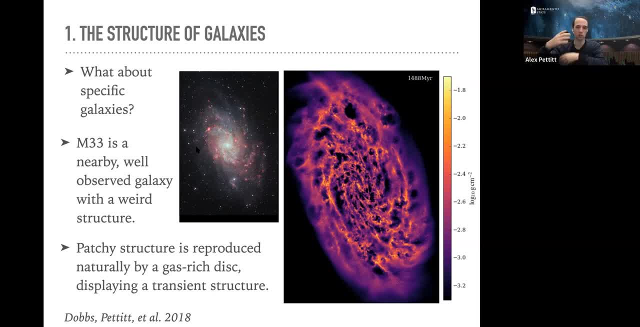 which moves the stars around as well, which helps sculpt the entire galaxy, And that's what we think is going along here. There's such a. The star formation is having such a strong effect because it helps build up that structure, which is quite easy to do. 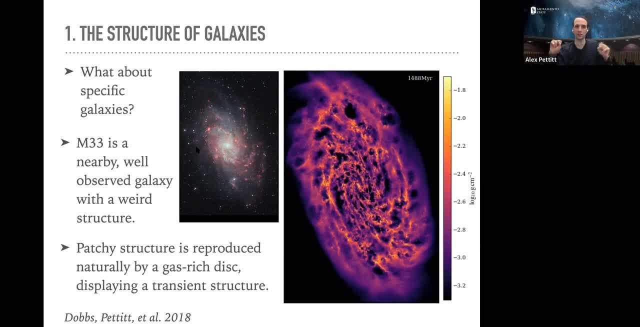 when the galaxy is quite small. When it's bigger it gets quite a bit harder for those effects to make a big difference. And we don't just look at And we don't just look at pretty pictures. So here is not just looking at the gas head on. 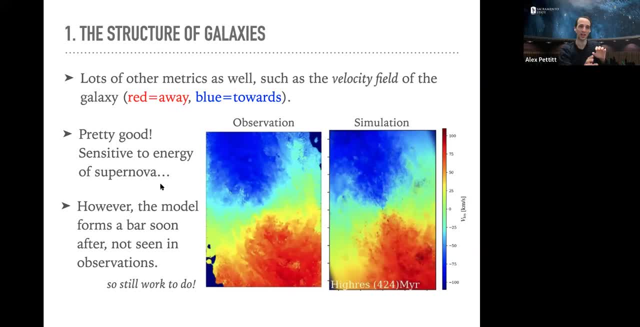 This is looking at features in the speed the gas is moving at. So the picture in the middle, these rainbow colors, show you differences in the speed that the gas is moving around in the galaxy. So negative is very blue, Positive is very red. 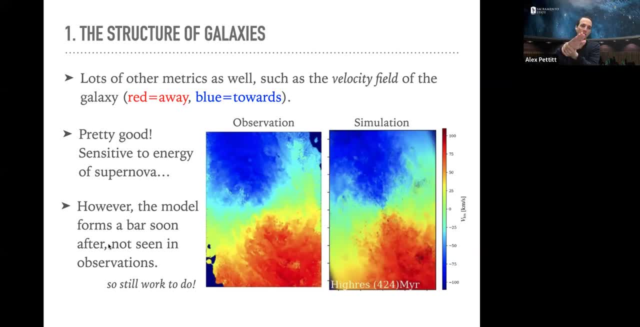 The galaxy is tilted a little bit. That's what gives it different colors. So the red stuff is coming towards you, The blue stuff is going away from you. So you can tell a little bit about the angle of the galaxy by looking at these maps. 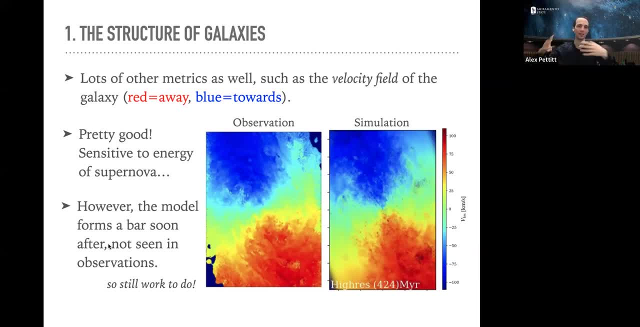 And the middle one is taken from a telescope. They've done some fancy spectroscopy and they've got these data out from the galaxy. But you see there's lots of features, right, It's not just a nice clean disk, There's lots of like fuzzy things. 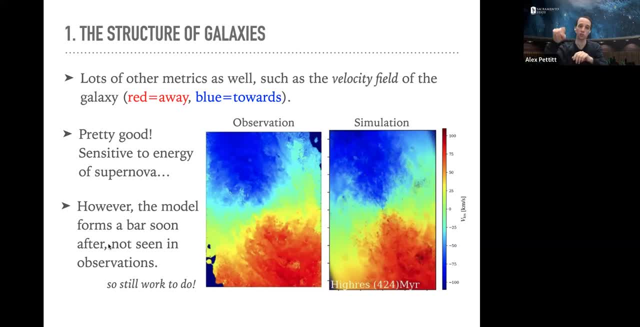 And lots of like wispy bits in there And there's a lot of structure in here. So when we made our simulations, this was kind of one of the tests we used: How well did we match this pattern If we made a galaxy where those green and red overlap regions? 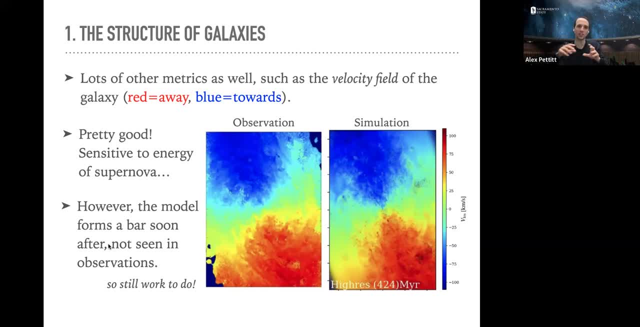 are very smooth, then we're probably not doing it right. So it was a nice little test bed to see if our simulation was reproducing the real thing or not. And this image on the right is the one from that galaxy I just showed you in the movie. 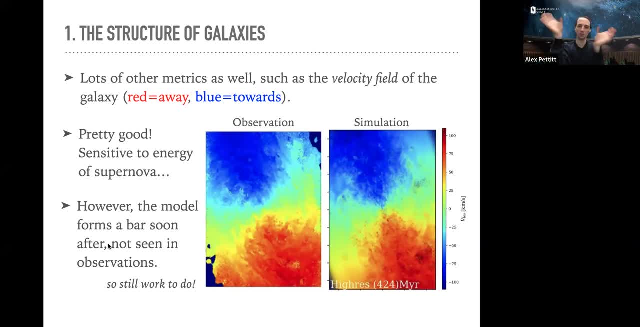 So it matches pretty nicely. So it matches pretty nicely how the differences in structure are in different radii of the disk. So this is an example of where simulators need to make sure they're doing the right thing, right. If we didn't look at this and it turned out, it didn't match at all. 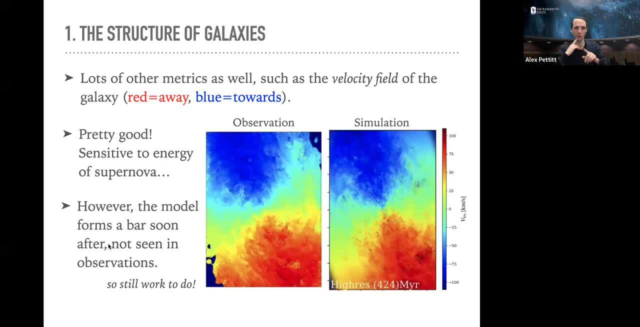 you'd have to stop and say to yourself: oh, why doesn't that work? What are we missing? Some physics or some assumption we've made? that means we're not getting the speeds of the gas right, which is probably wrong. I'm going to go back to the drawing board. 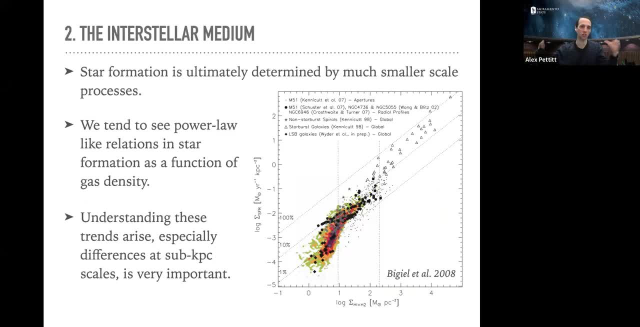 OK, So I've spent a bit of time talking about the structure of a galaxy. now We're going to delve in a little bit deeper and pick apart more of the smaller scale gas in a galaxy. So not looking at the whole thing, Dig down a little bit and try to understand more. 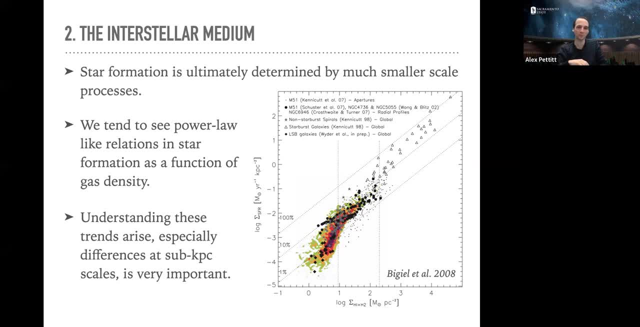 about what the gas is doing inside the galaxy. So galaxies like to form stars. right, I mentioned they were these star formation engines, But we want to know just a little bit more about how well they form stars. So why do some galaxies form stars better than others? 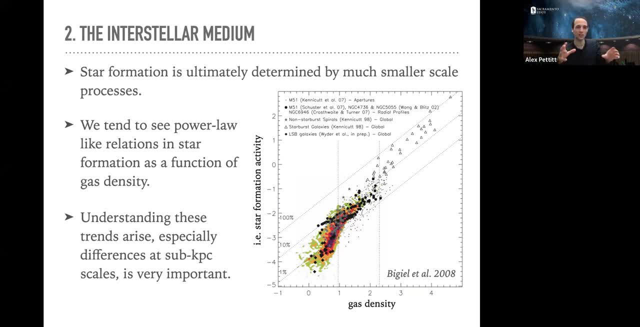 A very simple relationship that has been proposed in the literature is that more gas equals more stars, which kind of makes sense, right? If I've told you gas is the fuel of the stars, you'd expect if a galaxy, at a certain location, has more gas. 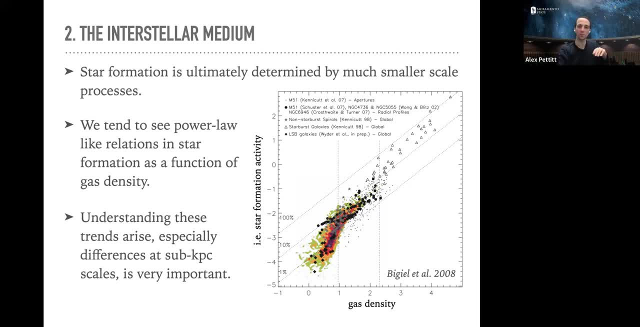 it will form more stars. This plot down here from Frank Bigiel in 2008, shows that relationship. So how much gas a galaxy has along the bottom, or the gas density, is technically what you look at. how much gas per unit area in a galaxy. 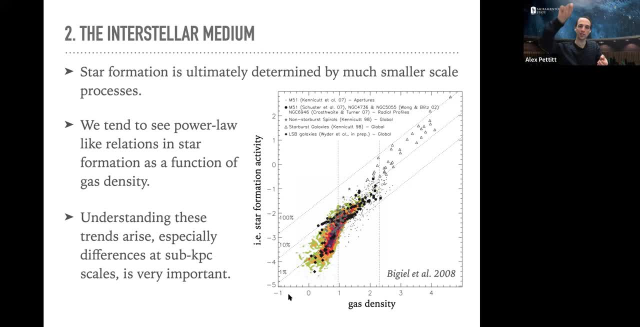 versus how well it's forming stars. So it's star formation activity on the vertical axis here. So how many stars in one year, in one patch on a galaxy does it form? Things high in the plot forming stars very well. Things low in the plot: 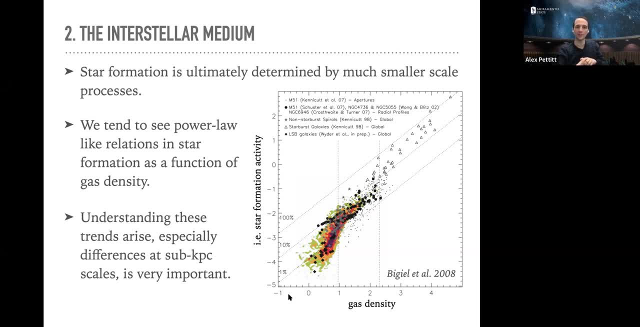 are forming stars very slowly or not at all, And all these data points on here and all these colors are different galaxies, different regions inside one galaxy, dwarf galaxies, very large galaxies, a huge collection of data here And you'll see it sort of matches-ish. 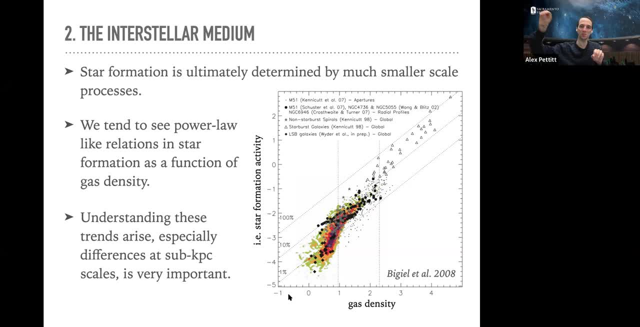 with a nice straight slope kind of. So it does seem to show that more gas equals more gas, More gas equals more star formation, which is sort of what we expect, But it's not super clean, right? You might have seen trends in physics. 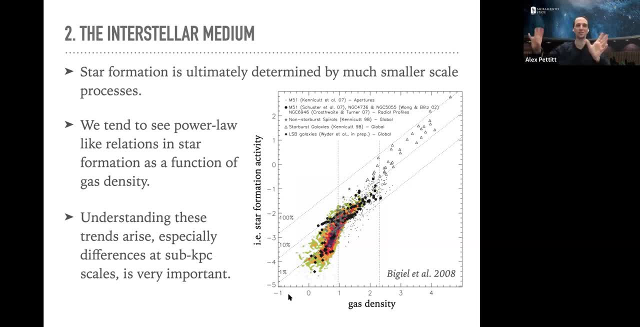 where you get a lovely straight line or you've seen like a black body curve from the universe. That's beautiful, Nice, clean line. This is a trend, but there's a lot of scatter right All along this line And at the bottom. 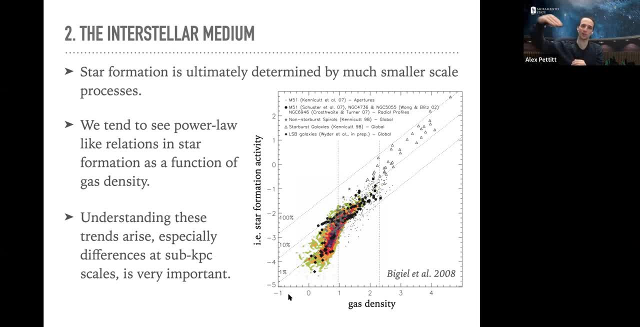 it also drops off the bottom end, Like it doesn't follow a linear curve even It sort of almost has like a bump as well partway up. So there's a lot going on here. It's clearly not just more gas, more stars. 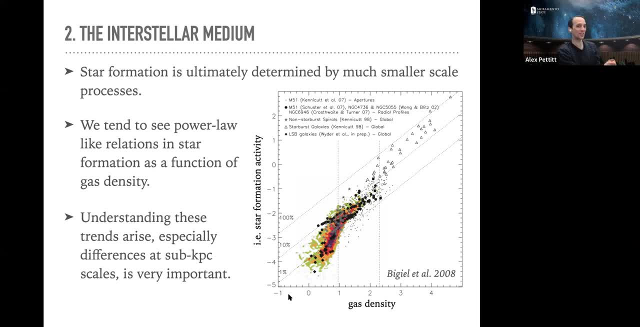 There's something else at play, At least one other thing. There's probably a lot of things at play changing how well a galaxy forms stars, So a lot of my work, especially recently, is trying to pick apart why some galaxies sit in certain parts of this relation. 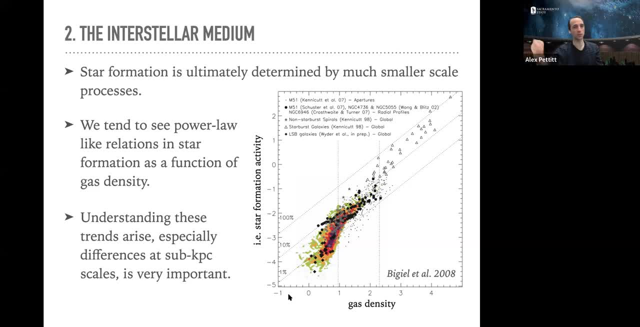 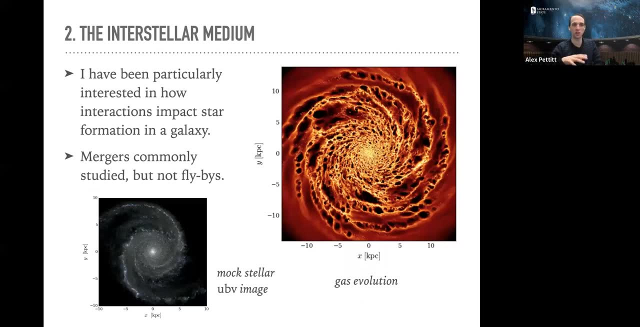 Why are some of them very good at forming stars? Why are some of them not good at forming stars? So, when I've been doing it recently and looking at interactions quite a bit, because interactions is what I like- this galaxy on the right here. 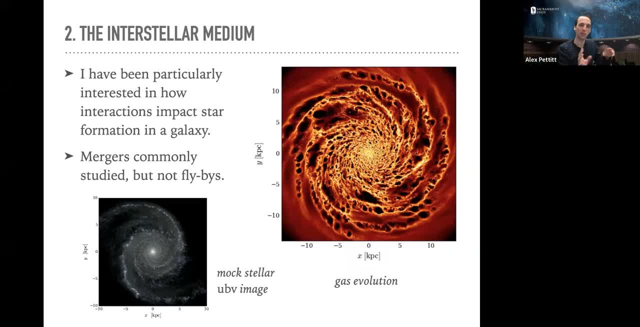 is similar to the interaction simulations I showed you earlier, but there's a lot more physics going on in here. So the galaxy is forming stars and those stars are spitting energy back out into the gas around it. So it's a bit juddery. 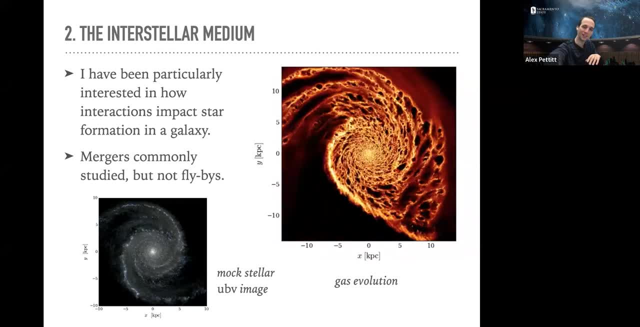 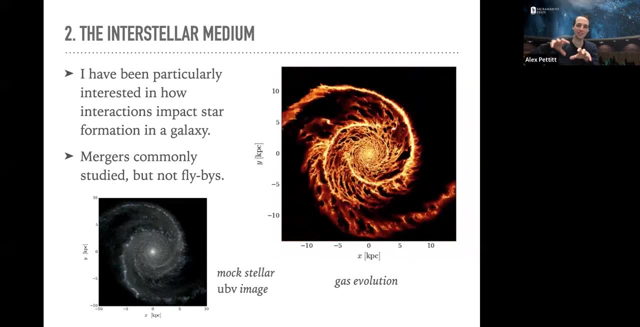 but you see the effect. The companion comes in from the right, goes down to the bottom, distorts it again, similar to before, but all the time in the background that you can't really see it is the galaxy is forming stars, depending on how it's changing in structure. 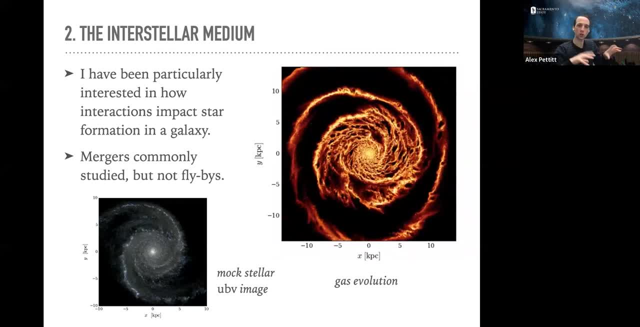 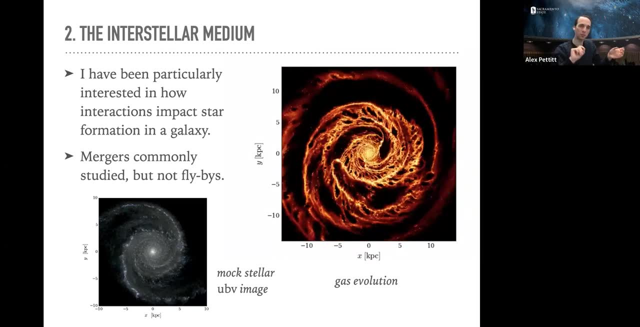 So the image on the bottom left here shows you the kind of thing that the Hubble Space Telescope would see. So these are the stars formed inside that galaxy and they're coloured by how massive those stars are or how young those stars are. So the blue patches are regions. 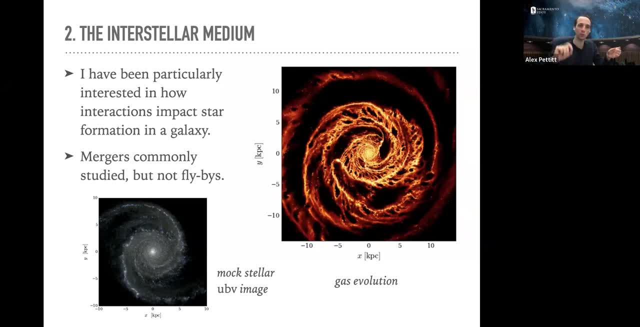 of very, very active stars and they're called star formations. There's lots of young blue massive things. The yellowy-reddy or yellowy-greeny parts are older stars. They haven't been formed very recently. They're a little bit older than the rest. 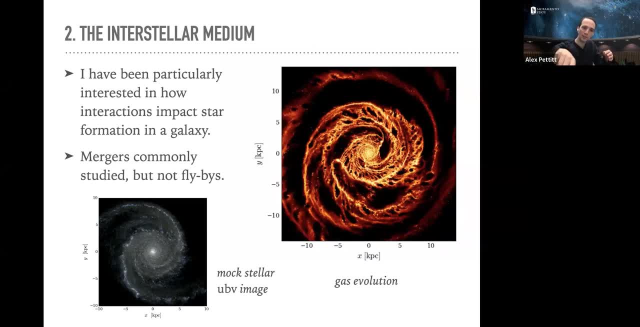 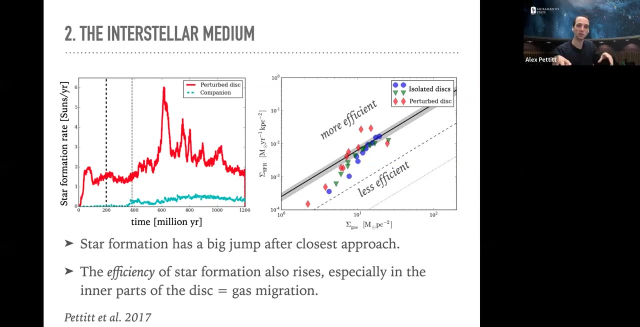 So you can see here all of the bluest stuff is right along the arms. These are the locations where we have the biggest amounts of density accumulated in one place, So that kind of makes sense. So this plot on the left shows the rate of star formation over time. 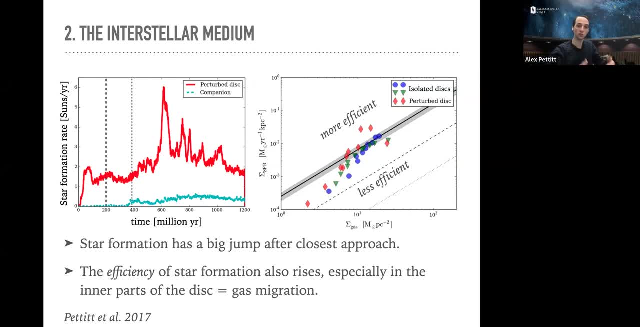 And the red line is kind of what you want to look at. So this is how many stars the galaxy has formed in a year. So on average, a galaxy will form one star a year. It's not a very high rate, but that's what the Milky Way does. 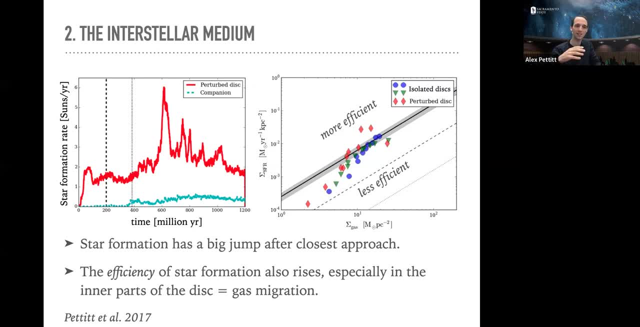 There's about one, one and a half stars a year that a galaxy makes, And this is the plot for that galaxy I just showed you. So it starts off about 1.5, one-ish, And when it spikes up is when the interaction happens. 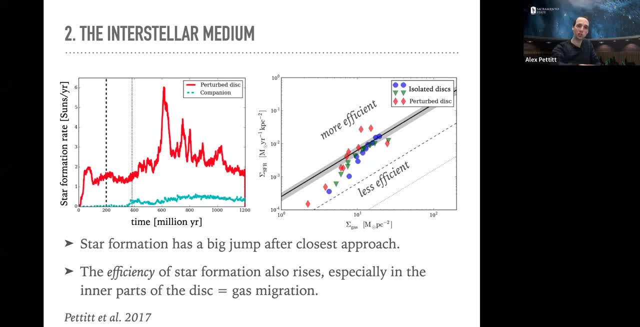 So the companion galaxy comes in, distorts it and we have this really big boost in how much stars the galaxy forms And it oscillates a little bit and slowly trickles back down to its value before the interaction. So the effect of being interacted with 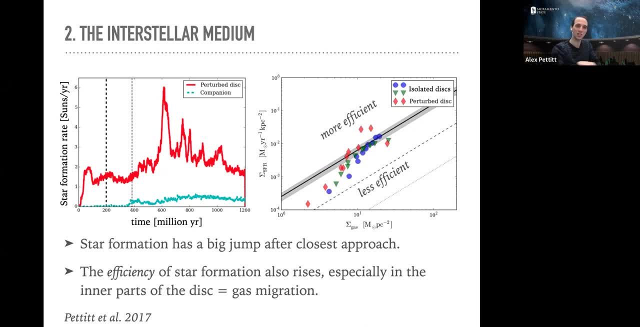 is clearly making it do something. in terms of its star formation. It triggers a burst of new stars. So as you give it a bit of a kick from gravity, it suddenly spits out a little bit of a lot more stars. You're helping it form more stars. 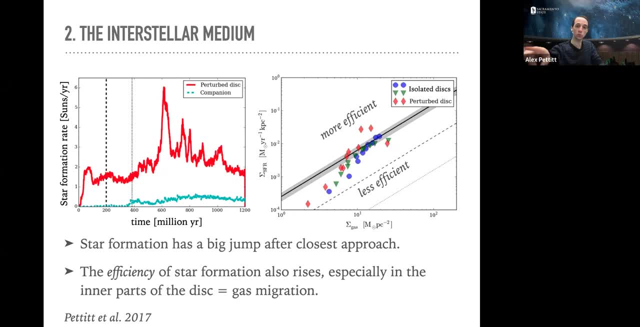 by interacting with it. The plot on the right here shows that amount of gas versus how much stars it's forming. That's the same as the plot I showed you from before, And the red diamonds on here are that interactive disk. So the red diamonds are the same. 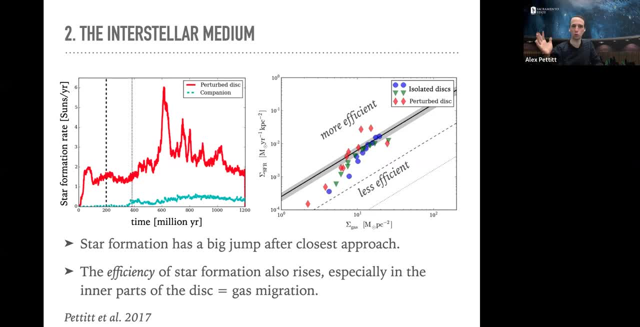 as the red line on the left, The blue and the green are for more normal galaxies that aren't being interacted with. And you see, that interaction causes those diamonds to peel up from that curve. Those red diamonds lie much higher, in the middle of the plot. 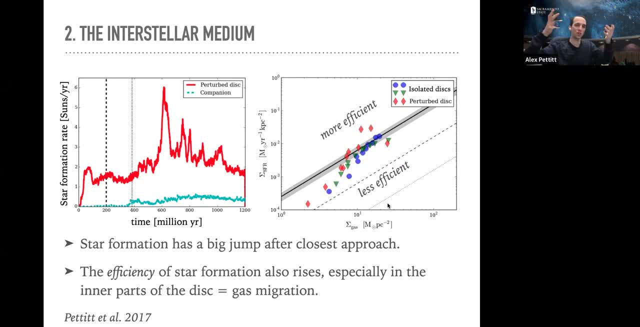 So by interacting with it, you are boosting its star formation activity. So we think that interactions with galaxies are helping them form stars a lot better than they would on their own in isolation, And there are some measurements of telescopes that begin to back this up. 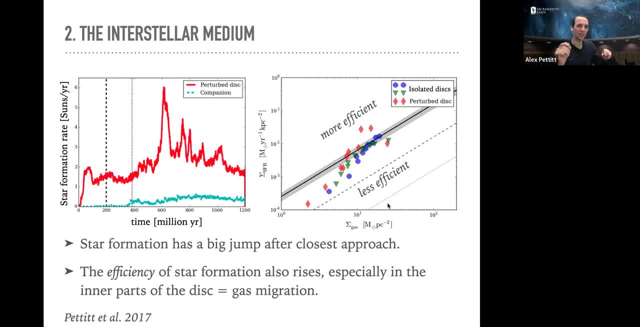 It's very hard to do to measure how many stars a galaxy is forming because you just have one image, right? How do you figure out how a rate of something from just one image is quite hard And you'd want lots of images, really, right? 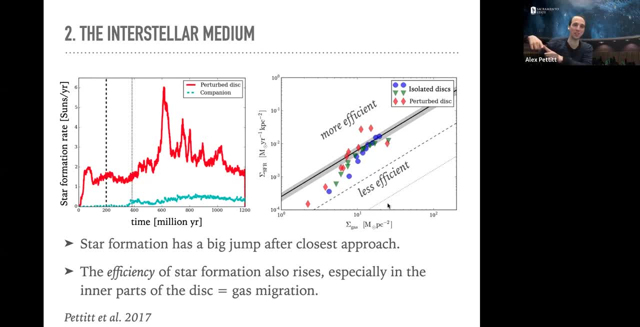 One now, one 5 billion years, one 10 billion years. That will tell you much clearer, But they can do it. It's hard, but they can get rough ideas of this as well And they seem to sort of agree that when galaxies are interacting, 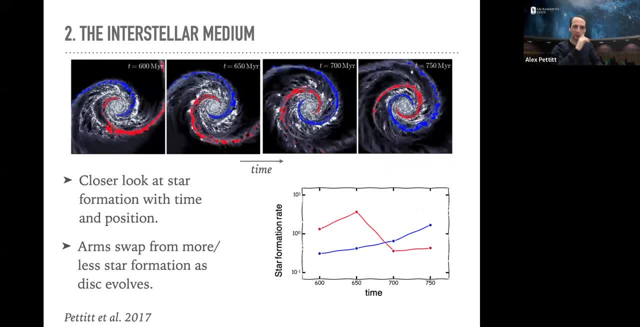 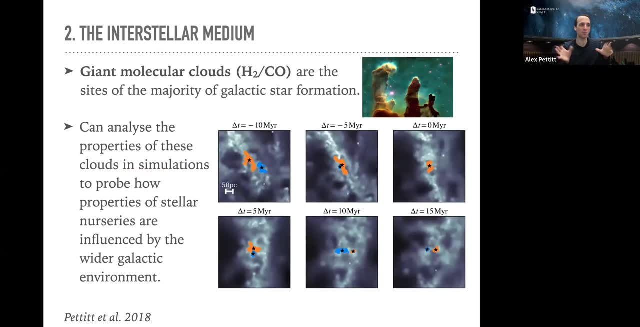 they will create more stars. This is a bit complicated to explain, I'll skip past this one. So when we talk about how a galaxy forms stars, I mentioned these cloud things right at the start, right? So a galaxy is a big accumulation of gas. 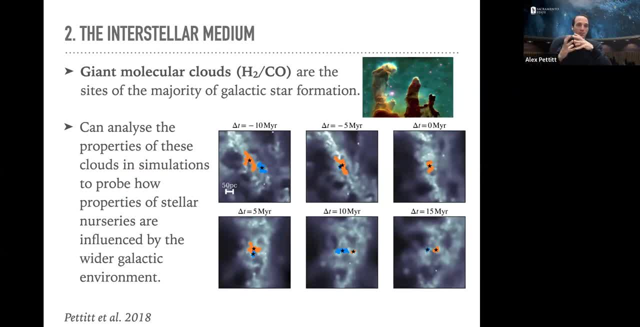 but the stars are formed inside big clouds inside them, So big gravitationally bound clouds of gas. We call these things giant molecular clouds. So giant because they're really really big. Molecular because they have lots of dense material inside them. So when gas gets very dense, very compact, 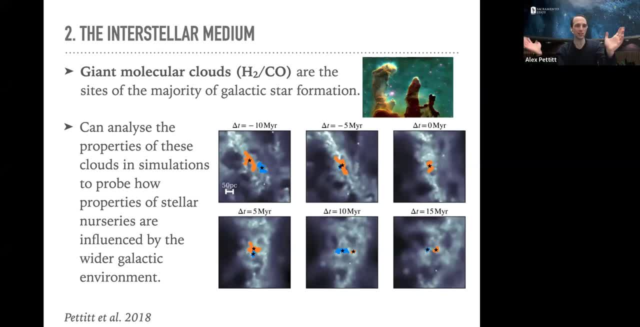 it will form molecules. Normally, gas in space is basically hydrogen or protons and electrons floating around. As you increase its density it becomes molecular, So you get things like H2, carbon monoxide- very famous interstellar molecules as well- And clouds, because they're big collections of gas. 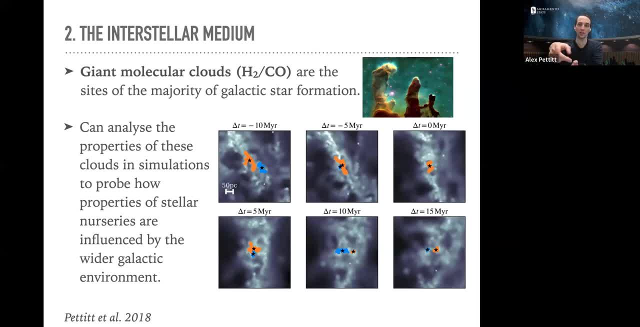 So call them clouds, right. So these huge things like the Pillars of Creation here, these are giant molecular clouds And they're basically stellar nurseries. They're the places where you're going to form your stars later on. So simulations have got good enough that we can kind of peer inside galaxies. 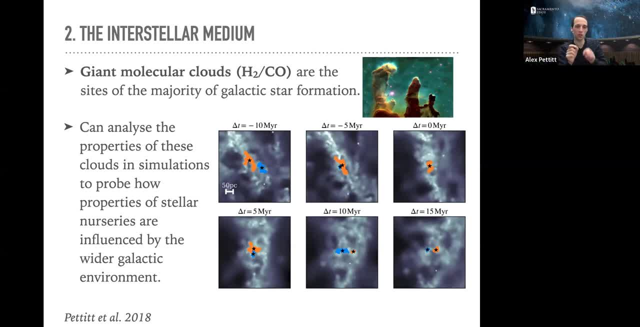 and measure this kind of stuff So we can look at the gas in there, do some fancy maths and find these clouds and study their properties and see how they move around. So these images on the bottom right here, the orange and the blue colours, show two clouds in a galaxy. 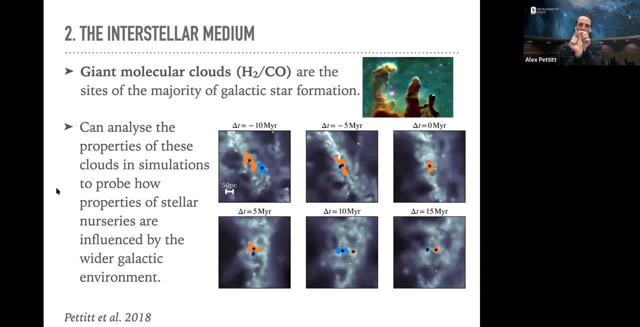 The patch is quite small. So on those movies I showed you, this is probably like a five by five pixel part of one of those galaxies. So it zoomed in really far And you can see these two clouds, the orange and the blue one. 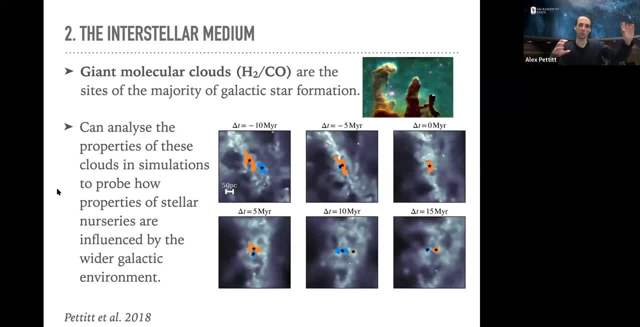 Time goes across and then, down across, Read it like a book. So in the blue and the orange they come together, They sort of merge in the top right and they split apart again afterwards, eating through their material as they go, and they get smaller and smaller in the process. 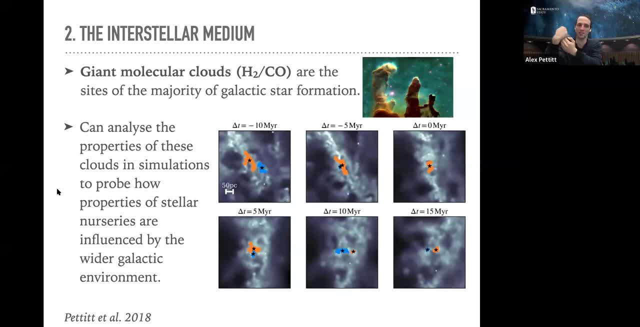 And it's called. they have a kind of collision right. They come together, collide, interact and then split apart. As you can see, the blue and the orange things move around compared to each other, And so we can study all the clouds in our simulations. 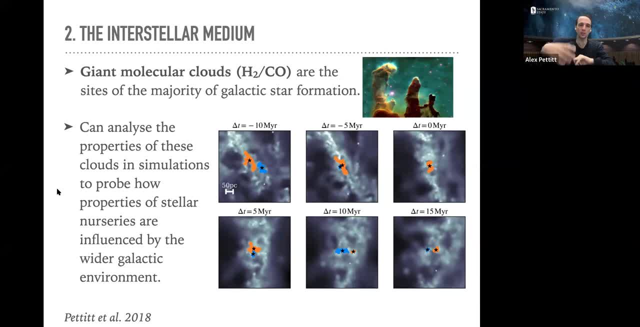 So I can look in and I can do this. This is two clouds, but the galaxy has about a thousand or so. When I open it up and pick it apart, you can measure about a thousand of these things And you can study their statistics, right. 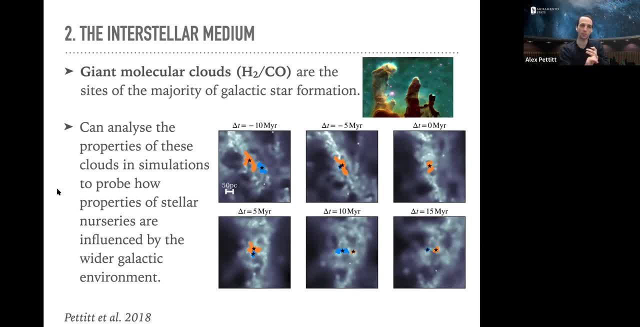 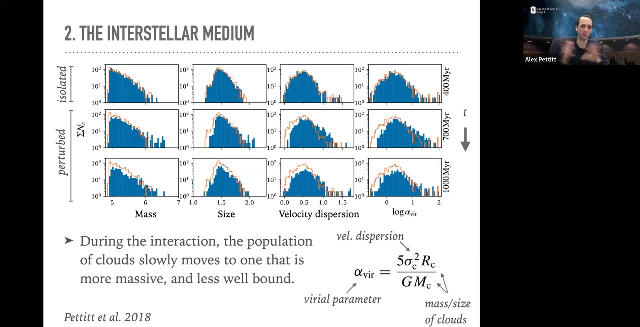 How heavy are the clouds? What kind of gravitational energy do they have? What kind of thermal energy do they have? Are they moving really fast? Are they so dynamic they're going to split themselves into pieces later on? Things like that. So these are some histograms showing the properties of those clouds. 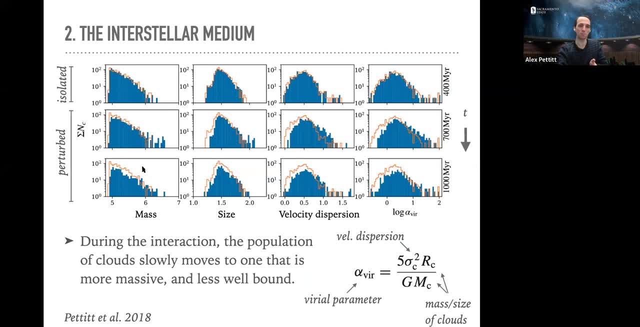 So this is probably going to be the last bit of science I'll show you, So I'll talk you through it. The plot on the left shows the mass of these clouds as a histogram And it's in log. So this is how many times the mass of the sun these clouds are. 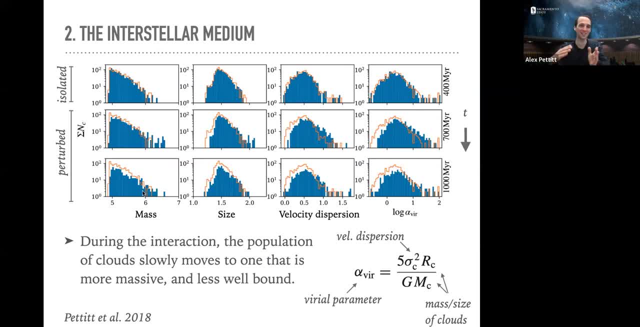 So they're pretty big: 10 to the 6 solar masses. You see, they're kind of pushed to the left, So there's lots of small clouds And it tails down to not many large clouds. So there's one or two with 10 to the 7.. 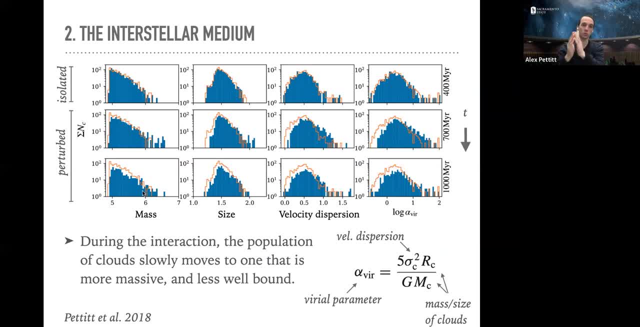 But most of them are 10 to the 5 or so. The next one across is their size, So their diameter. This is measured in parsecs. If you know a lot about astronomy, Don't worry about it. That just means the size of the clouds. 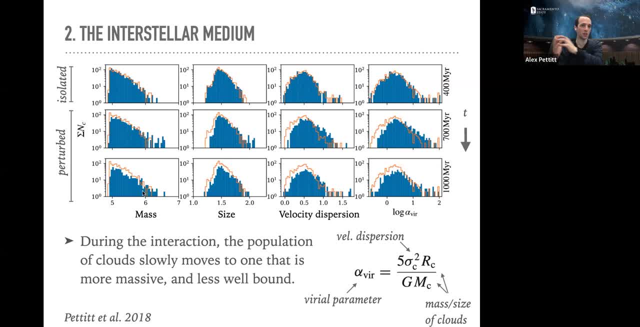 On the right is something called the velocity dispersion, Which basically means how much internal motion they have. If they have a lot of internal motion And they're whizzing around all the gas inside, Or if they're basically just inert And just sitting there not doing a lot, 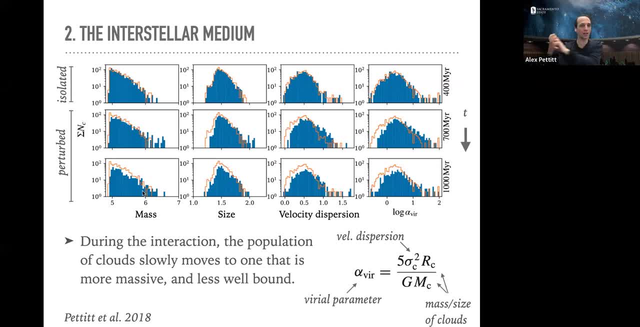 So zero means they're just nice and stable. The high numbers means they're very dynamic in their internal structure. And the thing on the right Is kind of a balance of all those properties, Because if you take a cloud's size, Its mass. 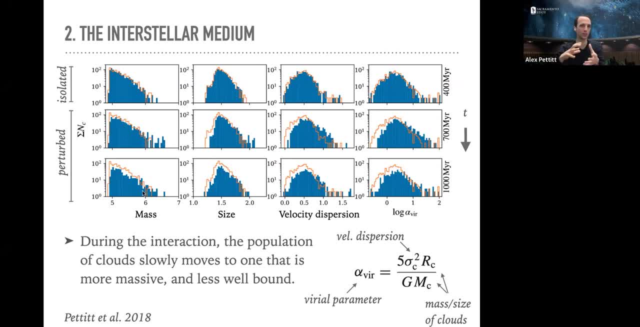 That tells you how gravitationally bound it is. Right. A lot of mass in a small size object, That's going to be nice and tight. Little mass in a big object, It's not going to be very tight at all. And the velocity dispersion tells you how fast that material is moving at inside. 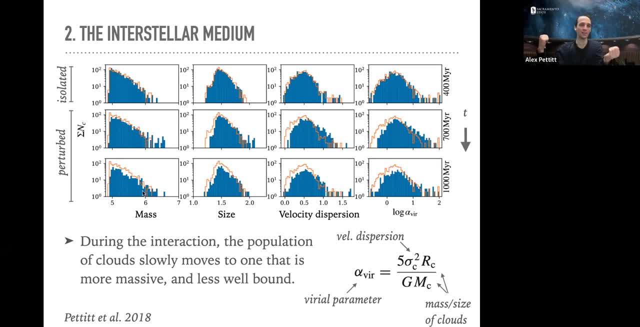 Which will tell you if it wants to rip itself apart or not. So there's a balance. So there's a balance between its mass, Its size And its internal motion That can kind of tell you how well bound that cloud is. So, this alpha thing, 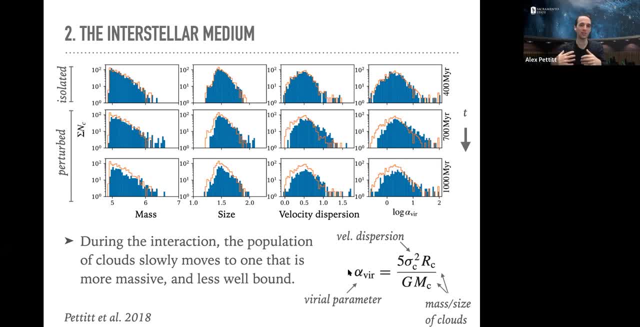 Is a balance between gravity And internal motion. So a low value means it's very well bound, It's very massive And it wants to keep tight. A very high value means it's ready to blow itself to pieces. It's got so much internal energy. 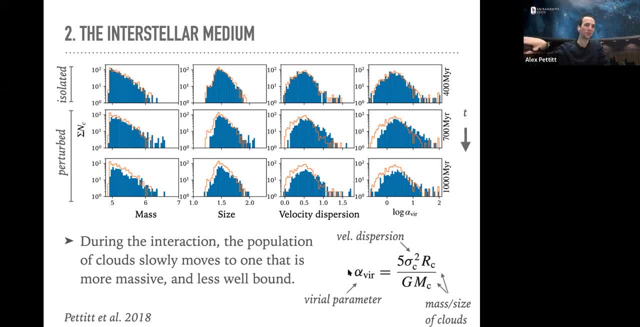 It wants to just break itself apart. So the important thing about this plot is: the top line shows you a galaxy on its own Sitting there, Not doing much, Being nice and isolated. The bottom two show you that galaxy after it's been interacted with. 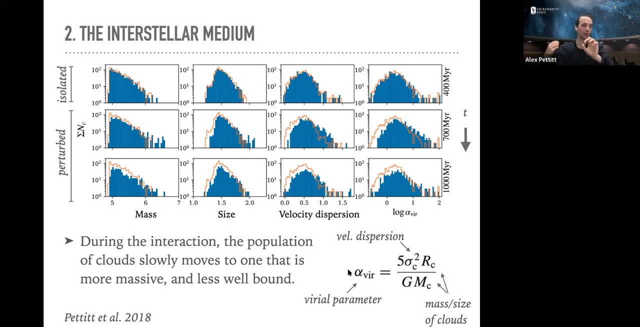 So you have a galaxy on its own And you have that interaction And the clouds all change. Some of the things change more than others. The orange line here in the bottom plots shows you the same stuff as the top row. So the orange line is the clouds when you aren't interacting with them. 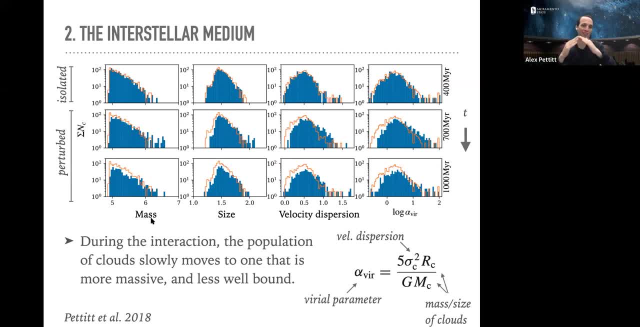 But when you interact you shift to the blue features. So the masses you lose some small mass clouds. But the important thing is the velocity dispersion. The third column shifts up quite a lot The orange versus the blue in the bottom lines in the velocity plot. 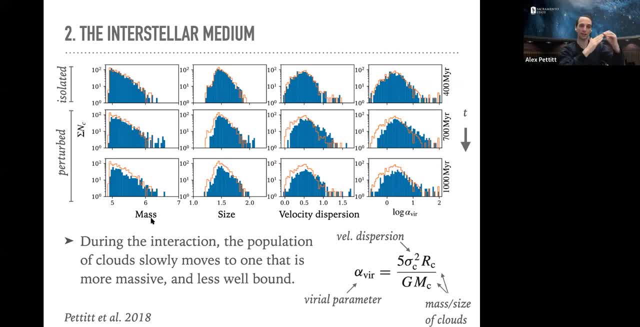 All shifts across a bit, Which is an impact, for that alpha thing Makes that shift up a bit, So all the clouds become a little bit larger And they're less bound due to this interaction. That extra energy you're supplying by the interaction is stirring up all the gas. 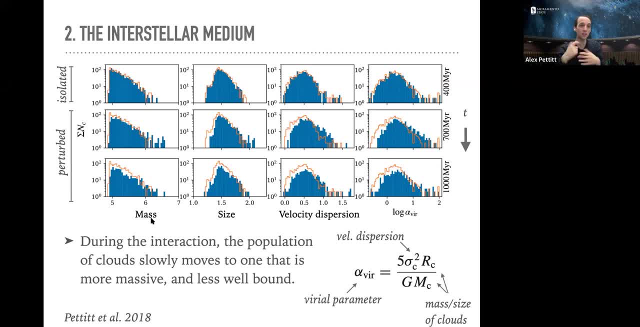 All the clouds are becoming much less stable And this has repercussions. If they're not very stable, they're going to want to form less stars. They're going to be less nice and quiet and ready to collapse. If you've made them all very dynamic, they're not going to want to settle down and form stars. 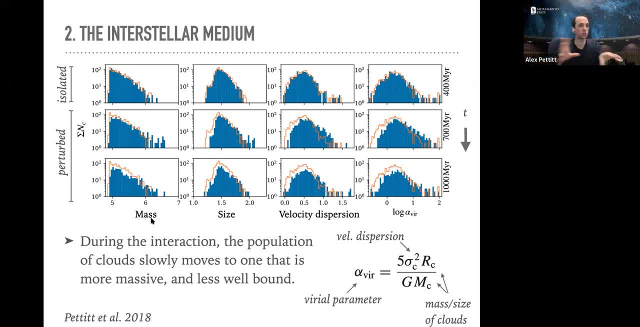 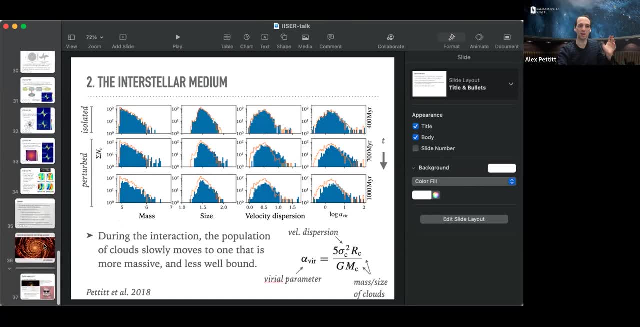 So this interaction is changing the clouds, Which is changing its ability to form stars later on. So I did warn that I might not be able to get to the third part of science, So I think I'll bring this to a close, I think. 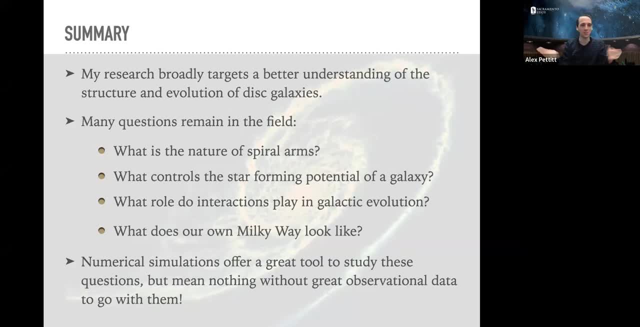 So I've talked to you a little bit about why I do what I do, How I do what I do, Where spirals come from- we think, Unanswered questions- And a little bit about the role of interactions, How they change what's happening inside a galaxy. 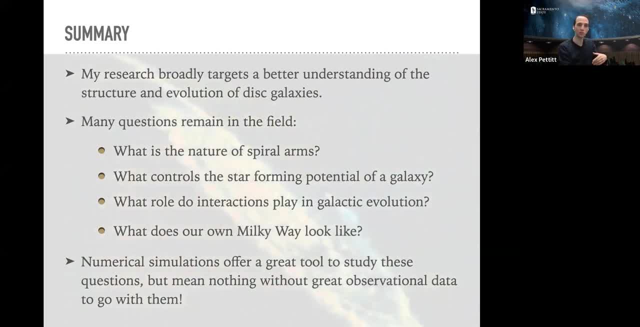 How they change its bar And how they change how it forms stars. I don't have a chance to talk about the final point here about the Milky Way, But if the authors, like I, can send them the slides for my talk And you can have a look yourselves. 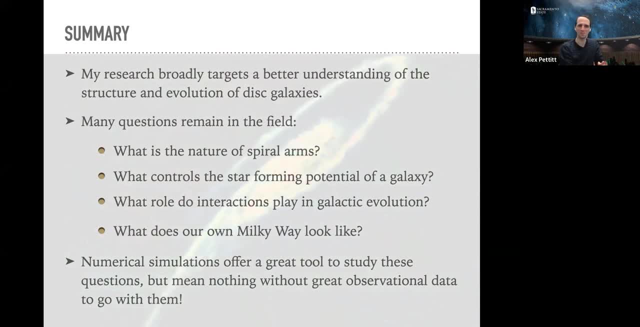 But yeah, thank you everybody for paying attention And I'll happily take questions for about eight or ten minutes max or so. So, thank you. Thank you so much for the talk. It is, I mean, it's- a chain that we could not complete. 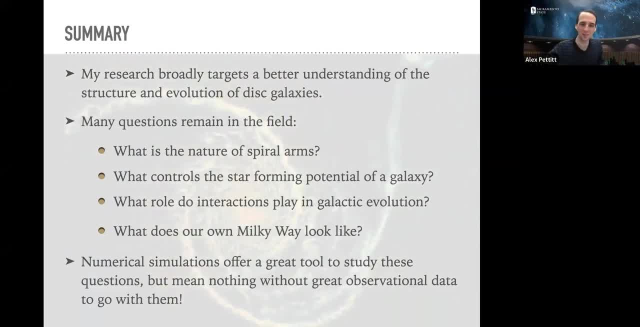 You know, do all the three things. Yeah, sorry about that. Okay, But if you have any questions, please raise your hand and ask them. If you don't, I have many, So you know. Okay, Abdul, you can unmute and ask. 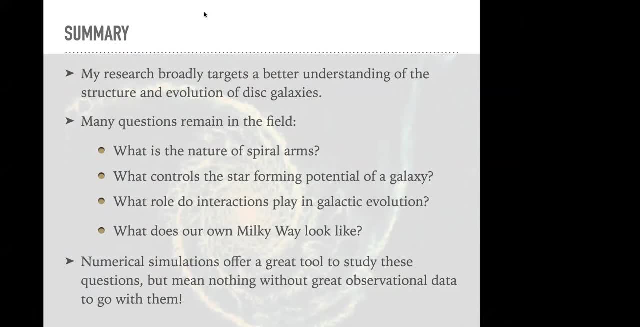 Hello Professor, Am I audible? Hello, Hello, Yeah, you're audible, Abdul. Yeah, I wanted to ask like that: Is there a relationship between like more dense galaxies, forms, like more number of stars, or it's nothing like that? Yeah, it sort of does. So the denser a galaxy gets, the more gas it has usually- And yes, it will normally form more stars. So the opposite is also true: When you have galaxies that don't have a lot of stars and don't have a lot of gas, they will be very inactive. 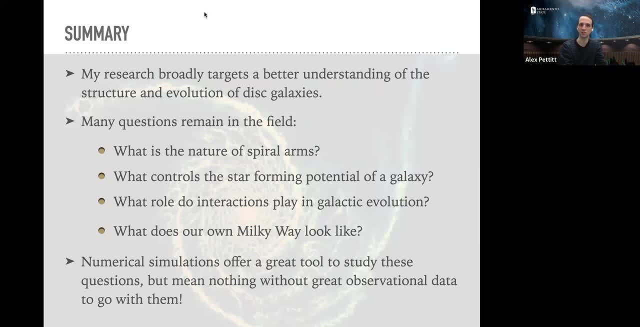 We say they're not forming many stars, They're very quiet. We'd say It's a similar kind of thing. And like one more question: like the same types of galaxies, like for example spiral galaxies, if they are like they have the same, approximately same distribution of, like gas mass, or that's not the case? like different galaxies, even though they're of similar type, they don't have like approximately similar type of distribution of gas masses, etc. 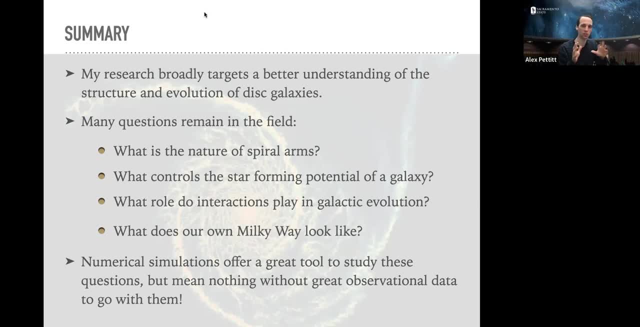 That's a very good question. So they all tend to have similar itch, So they all basically drop off. with radius in the center There's lots of gas And it all drops off as you get towards the edge which you expect. But there's differences, sometimes really big differences. 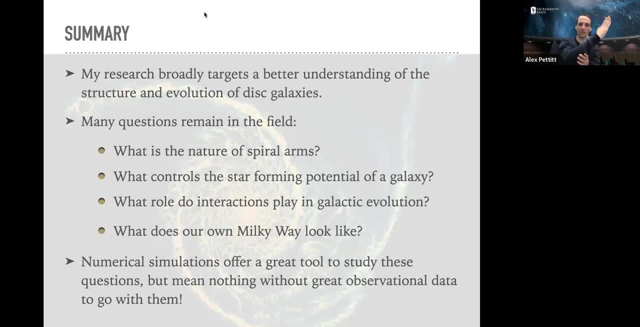 Like I showed you, one galaxy called Triangulum early on that dips and then gets really flat and then dips again. Some of them have bumps in them as well. So in general they all have a drop with radius, But some of them don't. 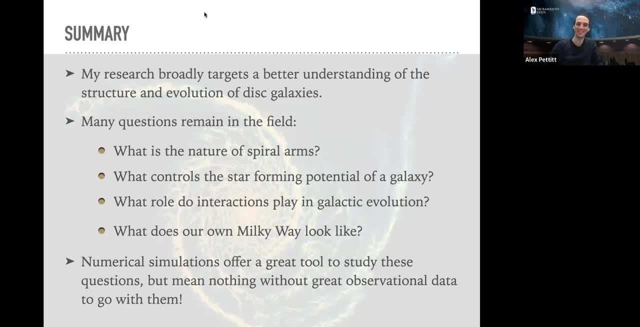 Some of them have very strange features And we don't know why. We're still kind of learning a lot about it. But yeah, good question, And I have to put that into my model. So sometimes I change how the gas is when I start to test these sorts of things. 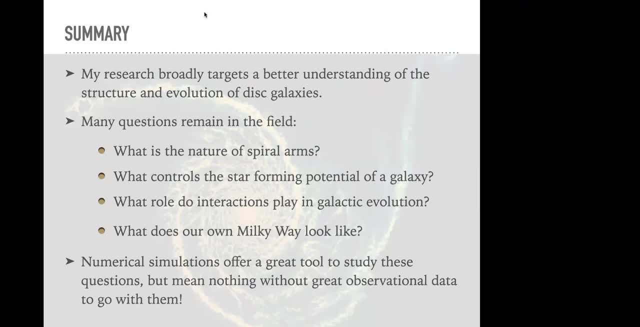 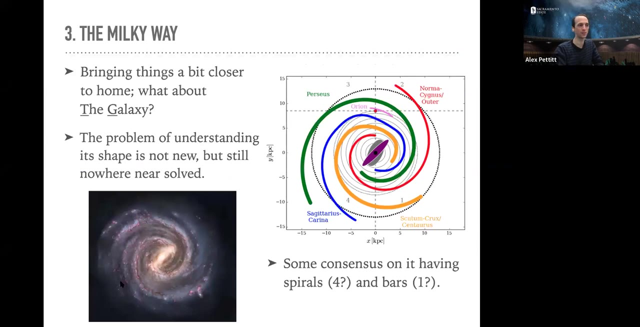 And final question Like this: is there, like what does our own Milky Way look like? I have studied like this: Isn't it like like barred structure, spiral galaxy? Yeah, we think it's barred, probably. I mean, if I flip back, we think it sort of looks like this on the bottom left: 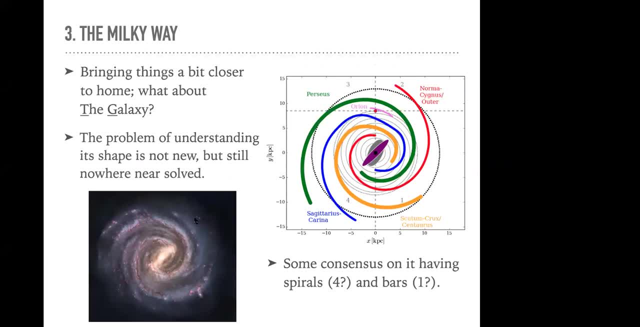 So there's a bar in the center as well. Sorry, I'm asking it: Is it still a mystery, Like we don't know, like we don't have observational values for it? No, no, totally It's a mystery. So there's a reason I put that image there and the other image on the right. 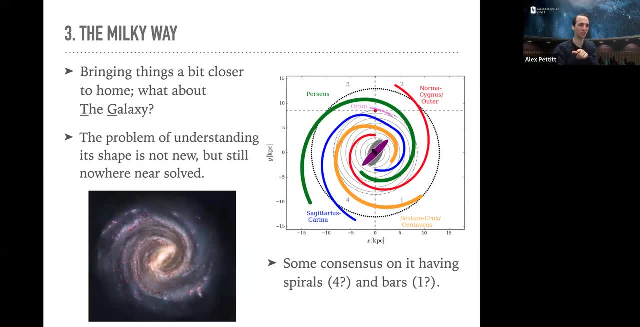 Because I think the image on the right is probably a bit more representative because there's a bit of unknown. We don't really know a lot of the features very well. With recent if you've heard of a telescope called Gaia that has, we think, actually seen the bar. 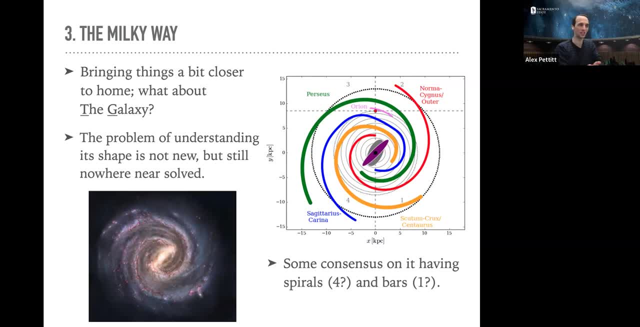 So for the first time we're pretty certain we can spot the bar and how many stars we count. We think Some people argue that the data is not good enough, But we are pretty certain there's a bar there. now It's just trying to find. everything else is quite difficult. 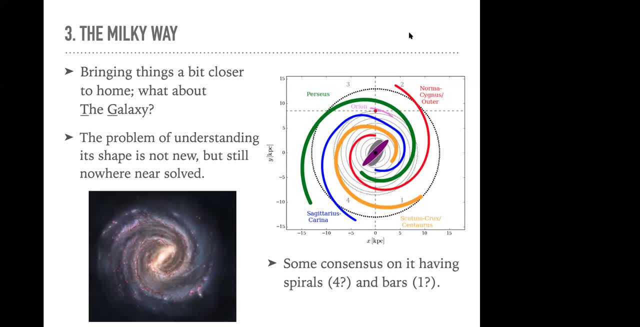 And one last, last question, Like: can we, through simulations, can we tell that whether a galaxy will result in the formation of planets or not? It's hard, People are trying, But to get that eventually we will. Right now not really. 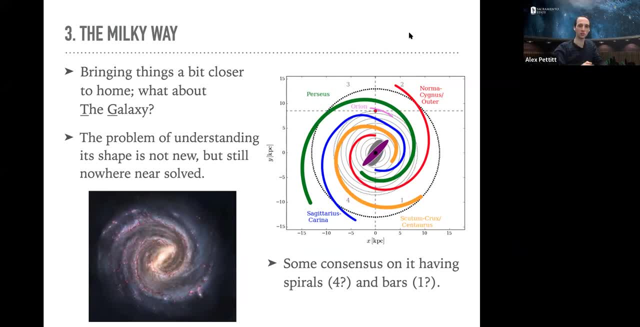 Because you have to go from such a large scale to such a small scale in your simulation that there's so many steps that have to be made. There's a lot of uncertainties. So eventually, but not right now- No, I don't think so anyway. 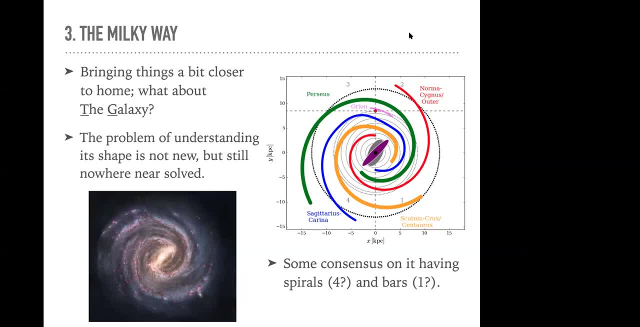 Thank you, No problem. Okay, So I have a question. When you say that you compare your simulations to experimental results, how exactly do you quantify when they are? you know when your results are, when the experiment is matching your simulation. 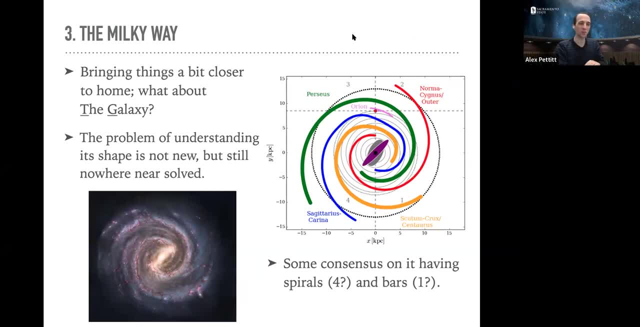 Well, that's a good question. So sometimes you do it just by like statistics, Like how many clouds have I formed compared to how many clouds a real galaxy has? Am I getting the magnitudes of how much velocity it has? right, for example? 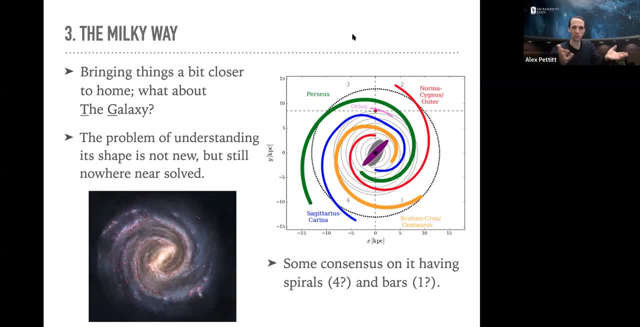 But sometimes you use a bit more sophisticated things like least squares fits or chi-squared fits, if you've heard of these things. Or some people use machine learning sometimes to fit it. I have not really tried that before, But some people do. 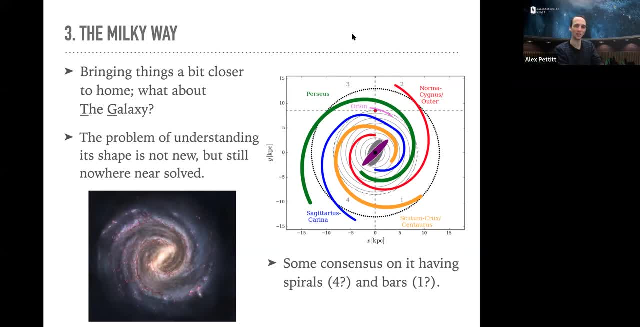 They'll test their galaxies, especially with the Milky Way stuff these days. They'll make a few models and they'll throw it at machine learning to try and get an in-between model between the ones that they've made. It's really interesting stuff. 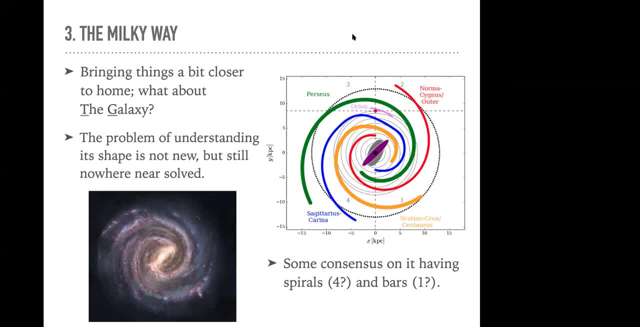 But yeah, we have a whole host of tools. we try, Right. And one more question. So when you said that there is a companion galaxy that interacts with another galaxy and that results in some, you know, very interesting stuff, So When you say companion galaxy, can we have a companion black hole, a supermassive black hole? 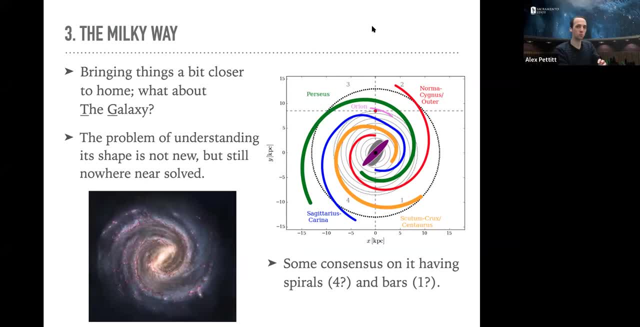 Is it at that scale, or You could, but it's very unlikely. So black holes, yeah, And we think it happens quite frequently actually that there's black holes that are around in our wide orbit of the galaxy, But to have a supermassive black hole, these only really exist at the center of other galaxies. 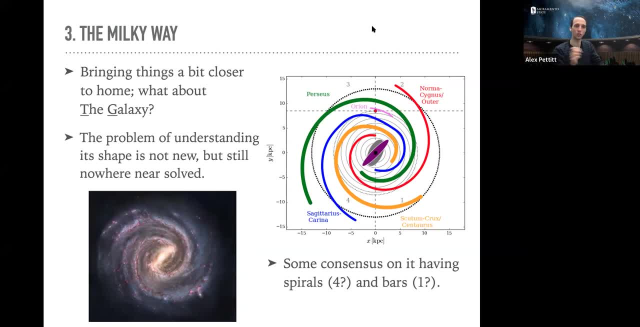 So to have one of those naked, as it were, would be very unusual. They normally have a whole galaxy around them, Right? Yeah, I don't know, Arhan, you can ask the question. I think, Actually, there's one in the chat which I'd like Alex to answer first. 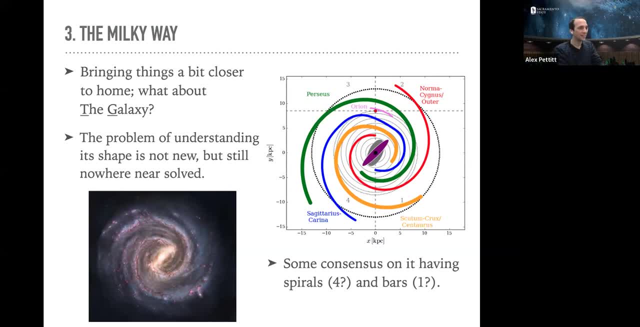 Okay, I'll have to take a second to read it. So yeah, the question here is what happens if not there's a dwarf and a big host, or if you've got two like Milky Way sized things and they interact, And normally this is really destructive. Actually this is more of a merger than an interaction, So I don't have any movies of it because I tend not to study it, because it sort of destroys everything And I'm more interested in leaving the galaxy almost in one piece afterwards. But yeah, when they're big enough, like roughly the same size, they will usually tell each other the bits and they'll fall into each other's own gravity and make one big chunky, usually elliptical afterwards. 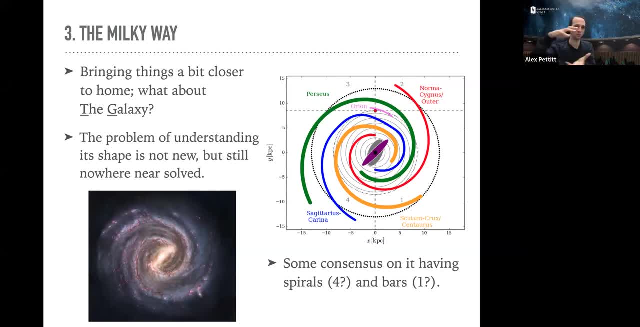 We talked about spirals here. There are other galaxies called ellipticals, which are kind of American football shaped and kind of boring because they don't have much gas and they're just red and very inert. Eventually, that is probably what the Milky Way is going to do when we collide with Andromeda in, you know, a few billion years from now. 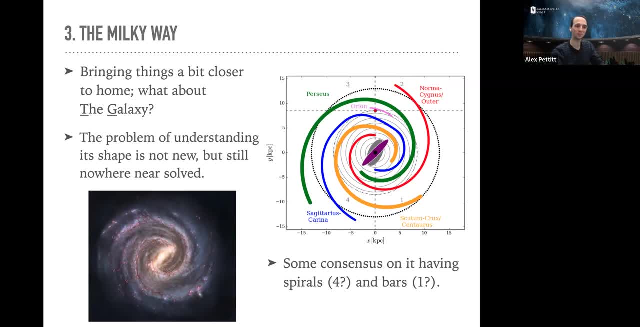 That's probably what's going to happen, because we have two very big galaxies coming towards each other. Good question, Could you scroll back to the star gas curve, Like the amount of gas in there? You know, in a galaxy, This thing. 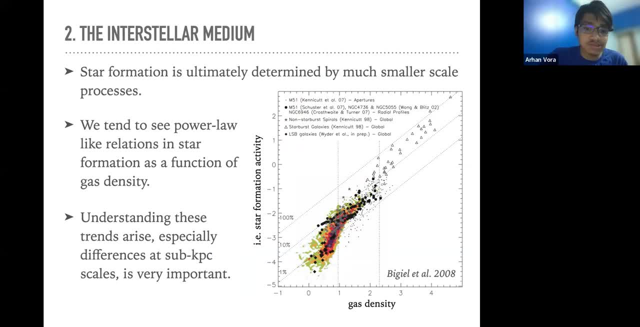 Yeah. So what's your like? what's your current hypothesis for why it takes a bit of time to start up? Is it that you know for star formation you need a special amount of gas? So maybe nobody agrees basically. 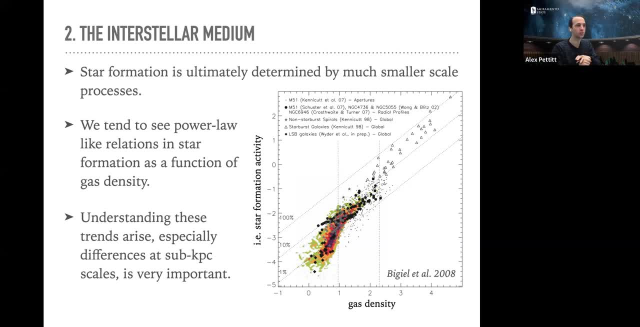 A lot of people think it's all to do with how well the galaxy makes molecules, because the molecular, the stage of forming molecular gas, is really important. When we look at this trend, It's much, much clearer if I just use molecular gas at the bottom. 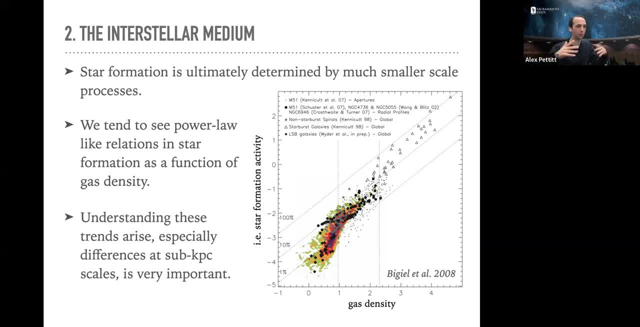 So right now it's all the gas in a galaxy: atoms, molecules, plasma. If you just make the same plot for just molecular gas, it's almost beautifully straight at the bottom. it picks it up quite a lot. So we think that transition is quite key, but that involves a lot of complicated chemistry. 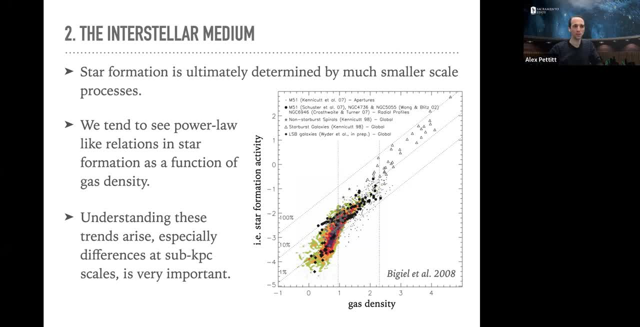 So the exact details aren't fully understood yet, But that's what people kind of think is going on. Okay, I think I maybe have time for one or two, because I do have to be somewhere shortly. I don't think I see any raised hand. 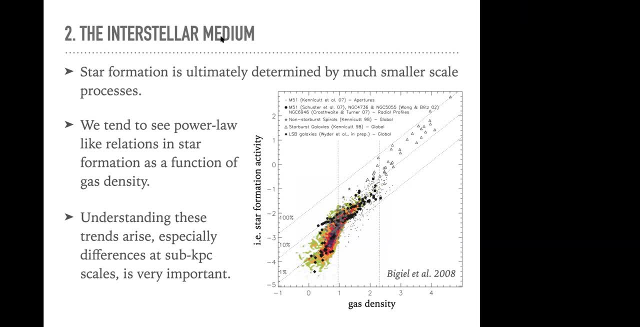 I have many questions so I can just go if no one else has questions. Okay, so when Shrey asked the question, if there are two oppositely oriented galaxies that collide, So is there some metric for angular momentum, like net angular momentum of the galaxy? 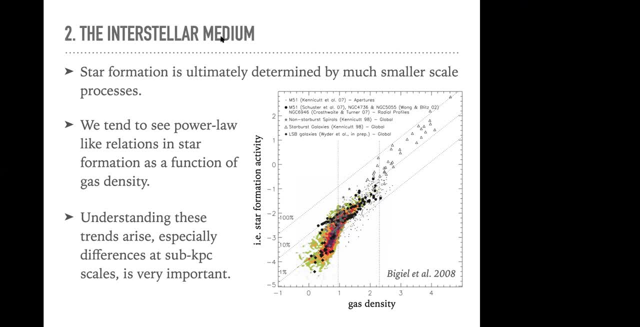 That sort of decreases when two oppositely spinning galaxies collide, Some sort of metric, I mean? there is a when they interact. there is a huge reshuffling about the angular momentum is right, Like when those, when the small companions comes past the big one, some of the angular momentum is imparted to the big galaxy. The companion normally slows down and its orbit decays and will normally get eaten by the main thing. So when you have two equal sized ones, there will be some rearrangement And it will depend on the orientation right, Like exactly where the angular momentum vector is pointing. 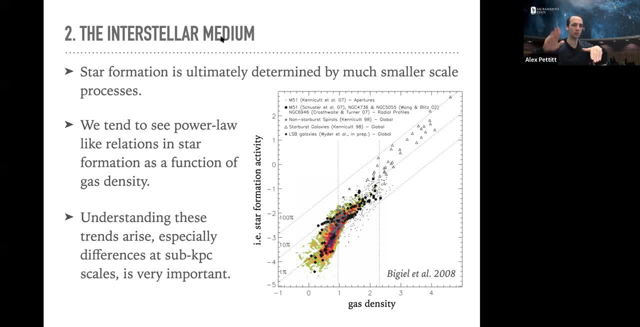 So I don't think there's one unified theory on the transport of angular momentum, because it's such a complicated thing, right? Galaxies in 3D space, in three orientations, with velocity vectors in 3D space, It's a it's a pretty complicated thing. 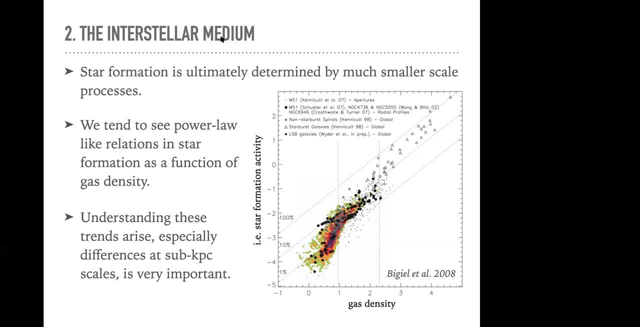 So it's not a feasible thing to calculate. It's a. yeah, it's like a, it's a. when you get beyond gravity of just two dots it gets really hard to do something about it. So it's really hard to do something analytically right. 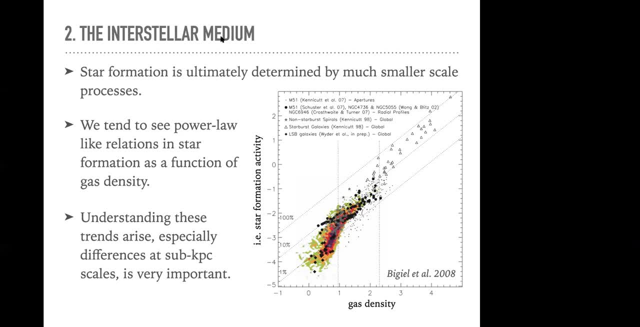 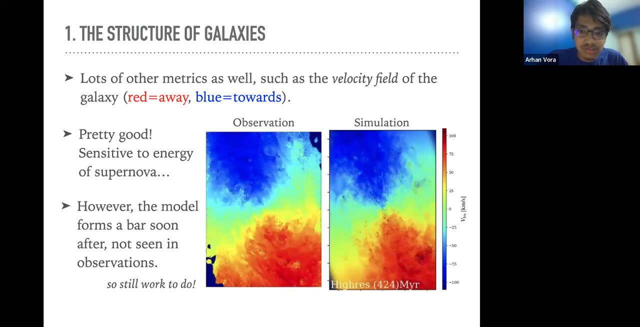 We've heard of the three body or N body problem. It's a. it's really hard, Right? This might have to be my last question. Yeah, That's fine. Could you skip back to the curve with the rainbow graphs, Like the ones where you had, like, plotted against a experiment? 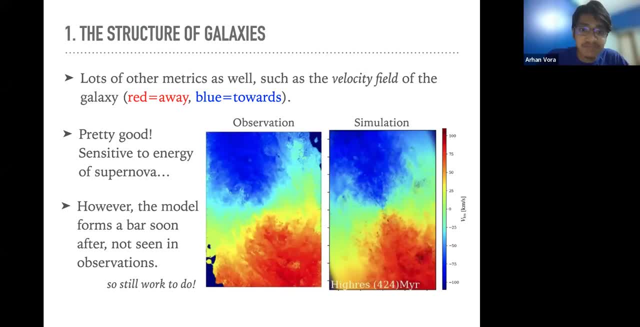 So there are these huge blotches in the bottom left corner of the observation which you don't see in the simulation. Oh yeah, That's just. that's just instrumental, Instrumental. There's no data there. basically, Their signal is so weak that they cut it out, because the galaxy gets really thin at the edges, right. 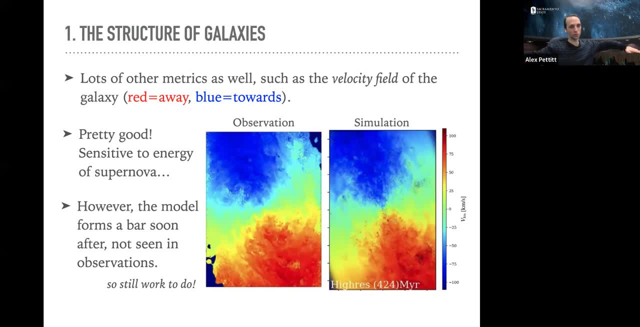 The amount of gas drops off from the center. So rather than have it very uncertain, they just cut out all the signal there. I see We have the same thing kind of. You see, in the bottom left, we run out of particles. 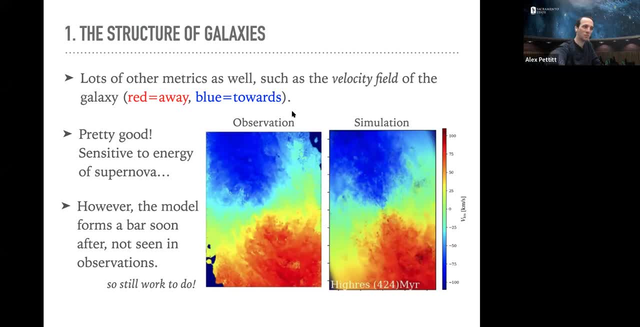 So my galaxy is so thin in the bottom left of my picture. on the right It's also dark blue, because I haven't got any resolution there either, I see. No, you wanted at least like regular, The other ones like kind of blotchy for some reason. 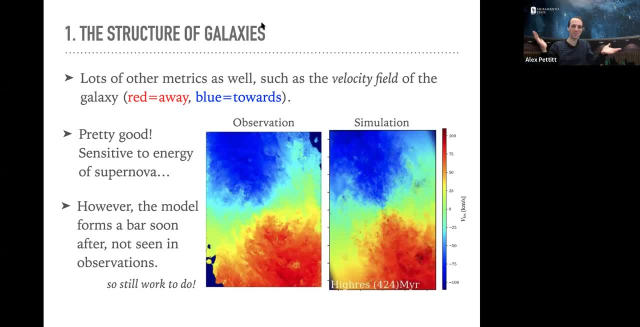 Yeah, Well, this is this is the, this is experiment. Experiment versus theory, right? Experimentalists always have problems with instruments and signal for noise It's always harder to control. Thank you very much. I guess I think we're done. 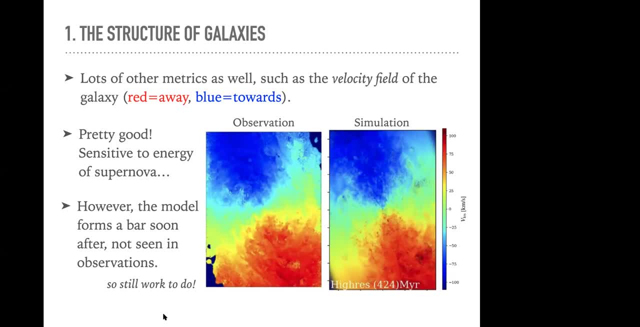 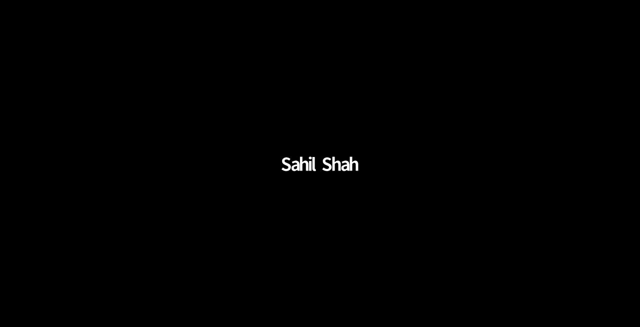 Yeah, I think so. Yeah, So thank you very much, Alex, for giving a talk. I mean, we have been trying to get this to happen for like almost a year, Two months now. Yeah, My apologies for getting timings mixed up, at least once. 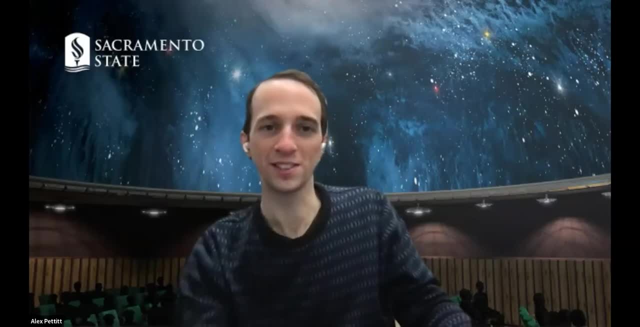 Yeah, I mean, but then I mean the talk was amazing And if you could come back again for for continuing and talking about the Milky Way, that would be amazing. So, Okay, Yeah, Maybe, maybe something for the future. 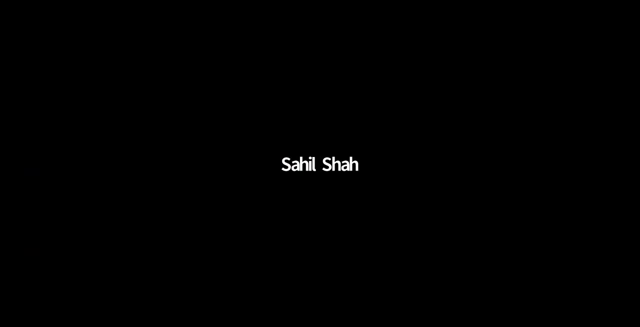 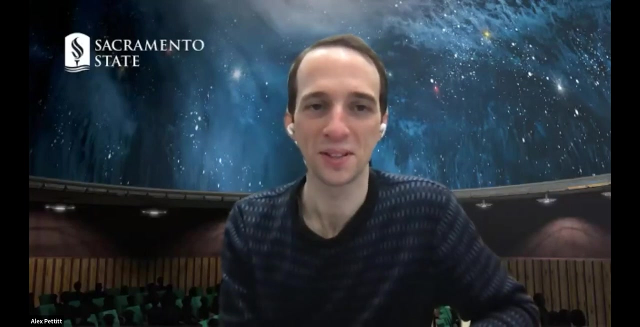